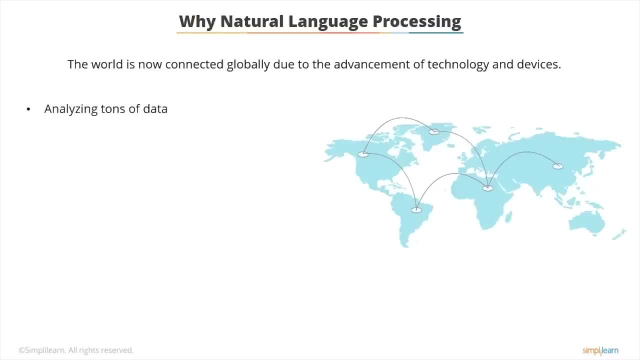 of challenges in analyzing data, including: analyzing the tons of data that is generated in the form of text, image, audios and videos, identifying approximately 6,500 languages and dialects followed across the globe. applying quantitative analysis on huge collections of data. handling ambiguities while interpreting data. 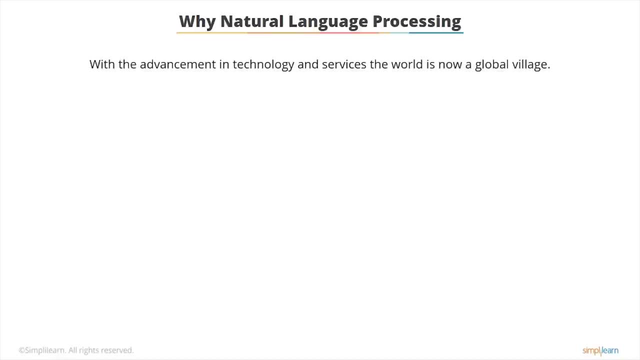 information. This is where natural language processing proves useful. One of the main goals of natural language processing is to understand various languages, process them and extract information from them. In NLP, full automation can be easily achieved by modern software libraries, modules and. 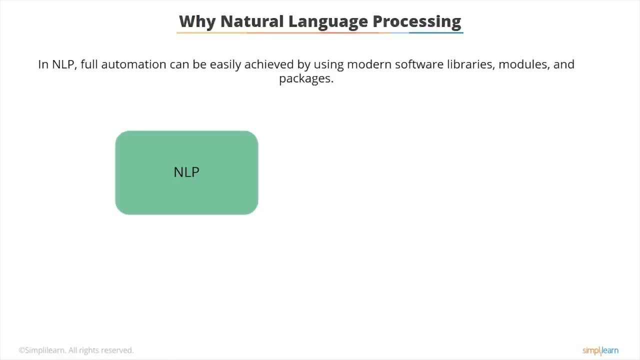 packages. These software libraries and packages are aware of diverse language and culture and categorize data accordingly, which enables them to understand and process various languages and cultures. This enables understanding sentiments better. With the help of these libraries, we can also build analytical models and automate. 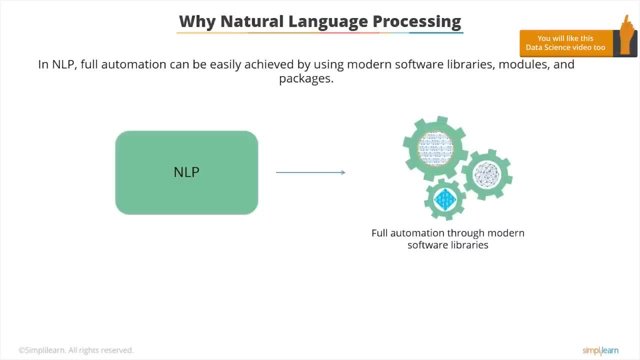 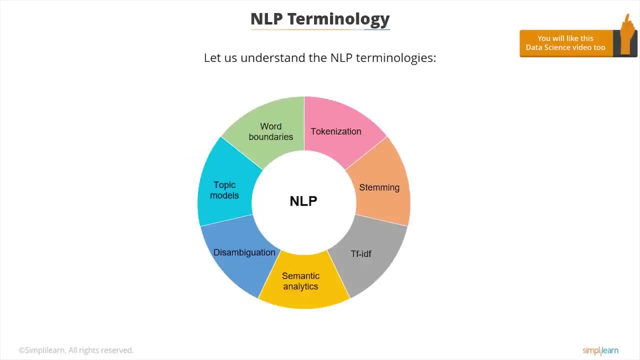 the natural language process with minimum or no human interventions. NLP Terminology: Now that you have understood why NLP is so important in recent times, it's time to make yourself comfortable with the NLP terminologies. 1. Word Boundaries: It determines where one word ends and the other. 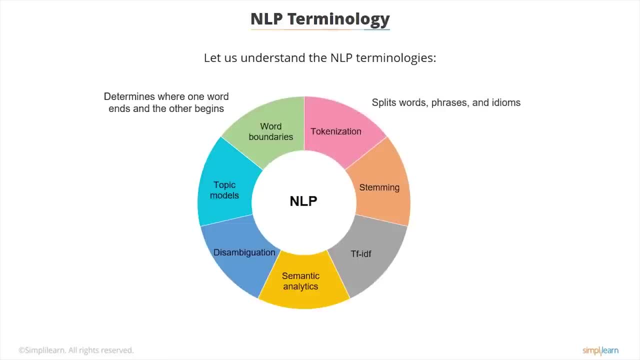 ends. 2. Tokenization: It's a technique to split words, phrases, idioms etc. present in a document. 3. Stemming: It's a process to map words to their stem or root. It's very useful in finding synonyms and extensively used in search engines. 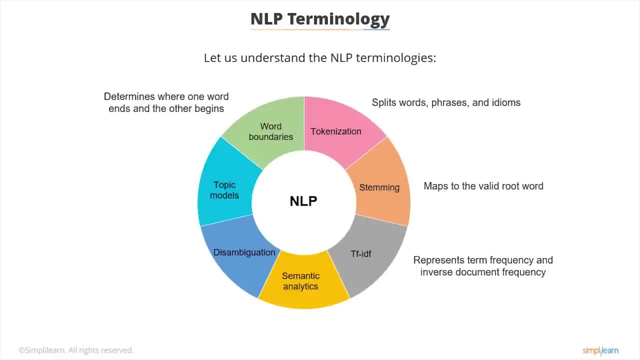 4. TF-IDF: It's a numerical value which represents how important a word is to a document or corpus. 5. Semantic Analytics: It's a technique in vectorial semantics of analyzing relationships between a set of documents and the terms it contains by producing a set. 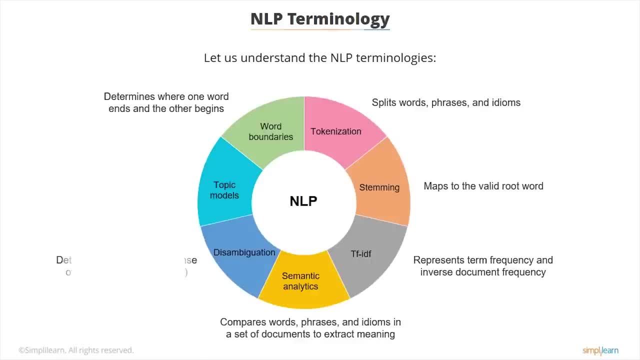 of concepts related to the documents and terms. 6. Disambiguation: It's a technique to determine the meaning and sense of words. 7. Topic Models: It's a type of statistical model. 1. for finding abstract topics which occur in a collection of documents. 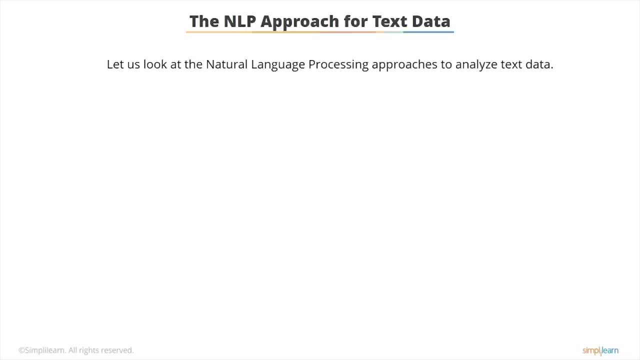 Now that you are familiar with the various terminologies, let's dive deeper into the NLP approaches to analyze text data. These approaches can be interrelated or they can be independently applied, depending on the type of data. to analyze Basic Text Processing: It's a way to analyze text and extract keywords. 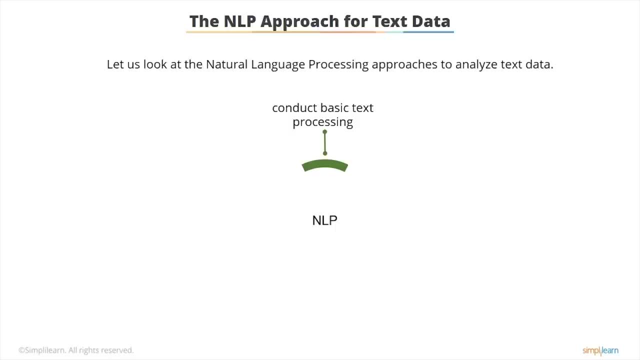 that sum up the style or basic context of the text, for example, if the content is religious or fictional. Categorizing and Tagging Words: This approach is about finding lexical categories and automatically tagging each word with its word class. For example, tag a word using languages such as Chinese, Spanish, etc. 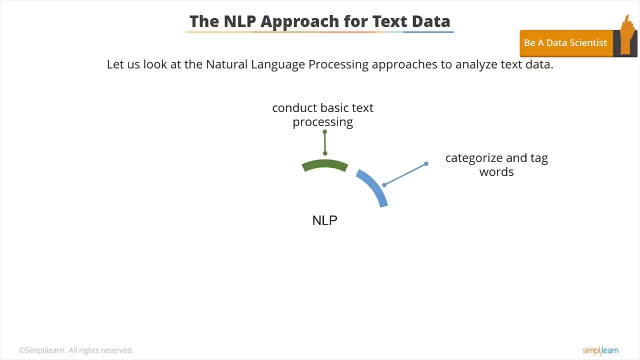 Words can also be tagged as adjectives, verbs, nouns and so on. Classified Text. With this approach, you can identify particular features of language and use them to classify it. For example, classify the text as sports, politics or technology. 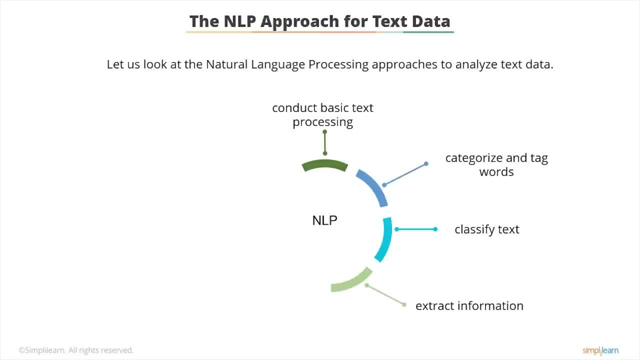 Extract Information: This approach is about identifying the entities and relationships in a text. to extract information in a structured way, For example, date, time, money and direction can be used to establish relationships with other words available in the text. the text. Analyze sentence structure In this approach, capture formal grammar to 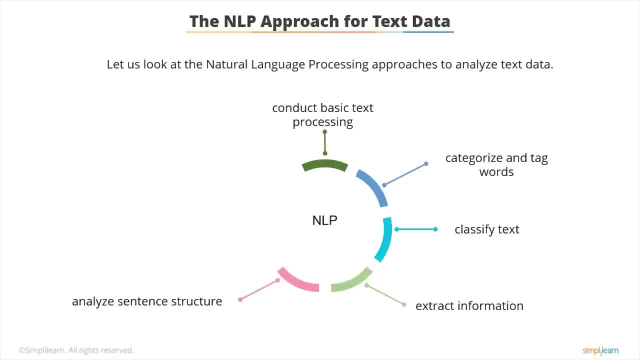 describe the structure of a set of sentences, For example. find a well-formed or ill-formed sentence structure. Build feature-based structure. Through this approach, we get an insight into grammatical categories of the text document. For example, detect features of text based on speech tag or some grammar. 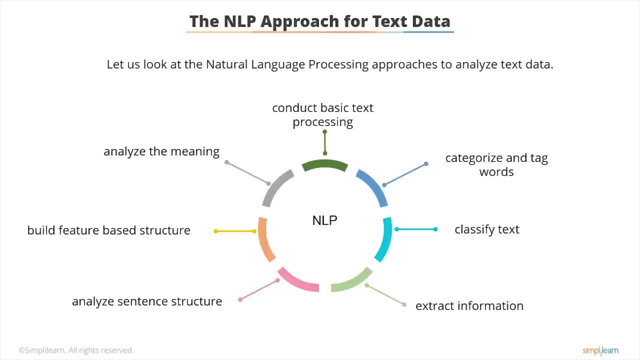 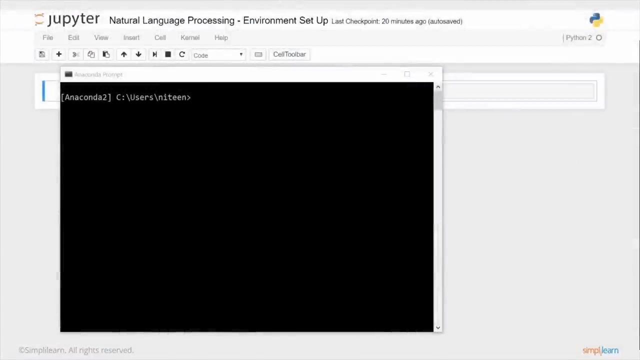 rules. Analyze the meaning, Perform quantitative analysis of the given set of data to extract the information. For example, find entities in the text and try to establish a relationship between them. In this demo, we'll view how to install NLP environment. Let's open the Anaconda. 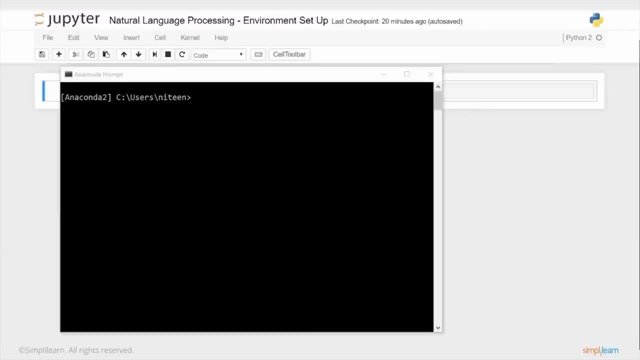 prompt. Please ensure that your system is connected to the Internet. In this demo we'll view how to install NLP environment. Let's go ahead and enter conda: install scikit-learn. It will install the scikit-learn package Enter. 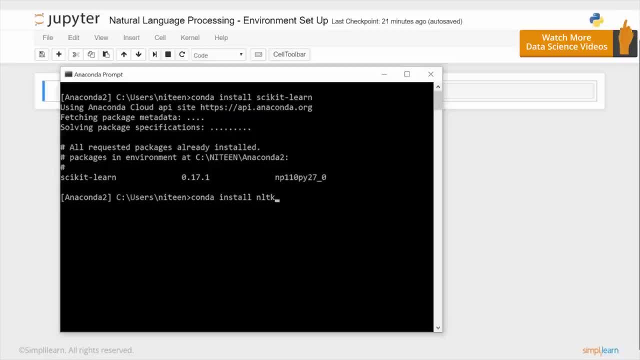 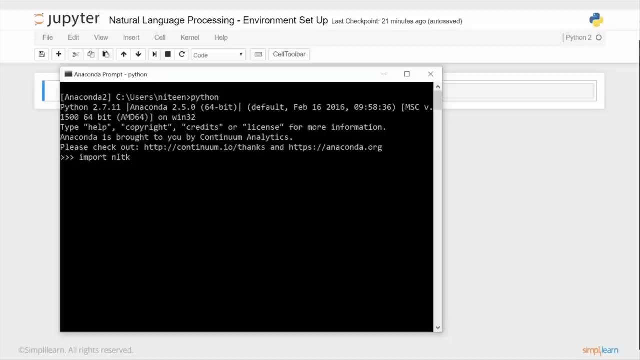 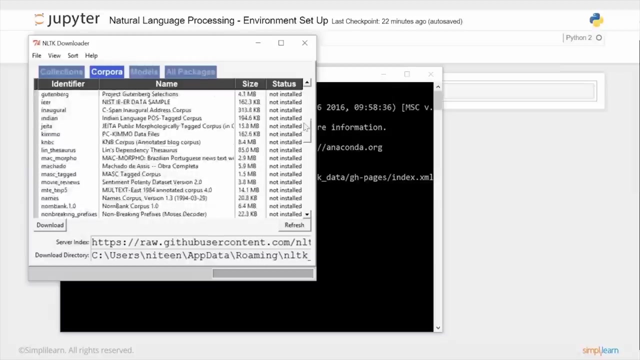 conda install nltk. It will install the nltk package into your Python environment. Now type in Python in Anaconda prompt command line. Type in import nltk- here to install the corpus collections and models. We are interested in installing StopWords corpus. Select it and then click download. 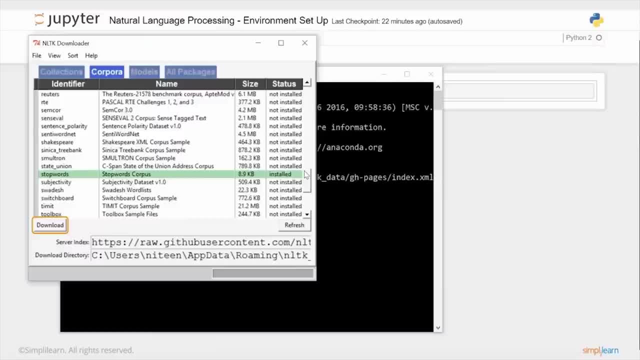 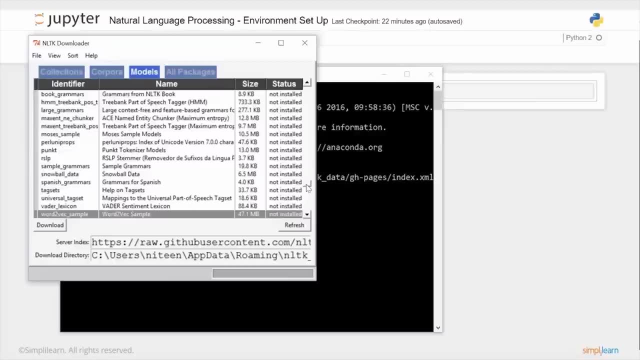 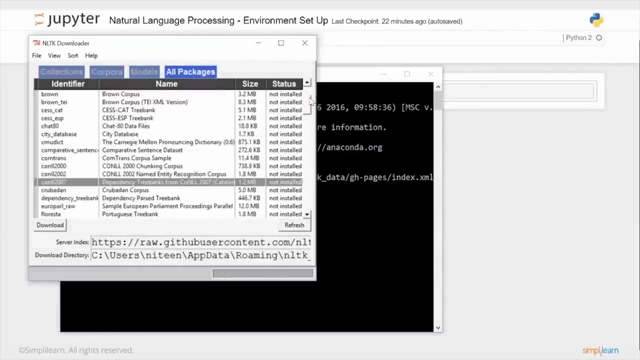 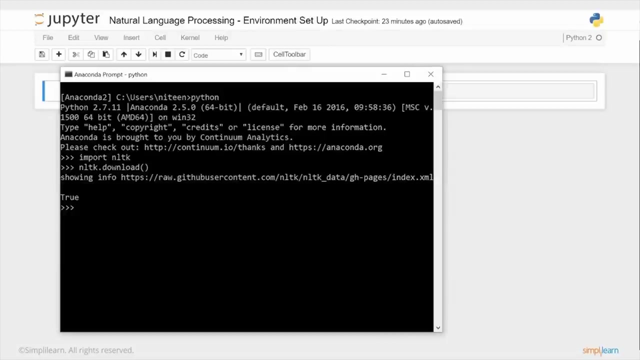 button. It will install the StopWords corpus in your Python environment. Now let's navigate through the other models and all packages Ensure that StopWords status is installed. Now you can close the window and go back to Jupyter Notebook environment. In this demo, you learned how to install the NLP environment. 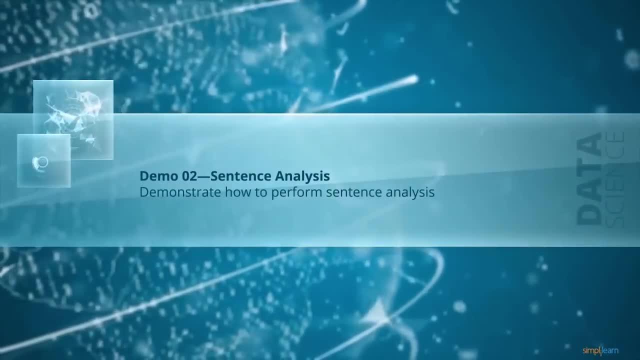 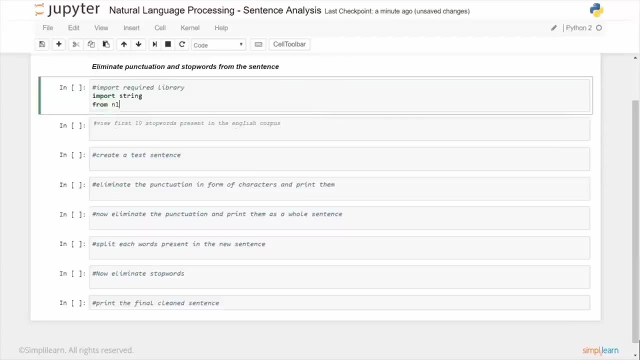 In this demo you'll learn how to perform sentence analysis. Let's start by importing the required library class string from nltk corpus. Let's then import StopWords, which we've installed earlier as part of the environment set up In the world of text analysis. stop words usually have little lexical meaning. Some 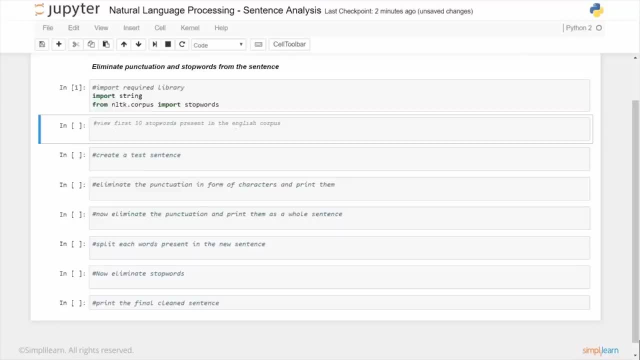 examples of StopWords are I, me, myself, we, our, ours, you, yours, and their Stop words usually have little lexical meaning. Some examples of Stop words are I, me, myself, you, yours, and so on. 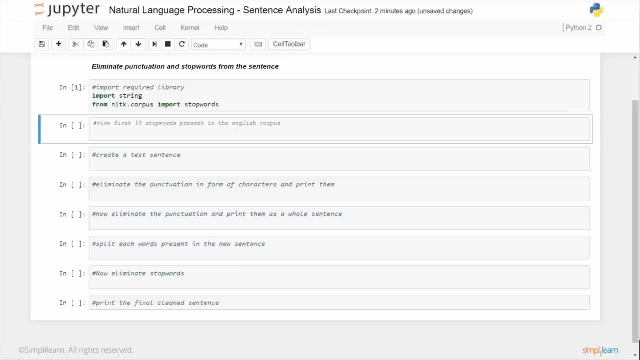 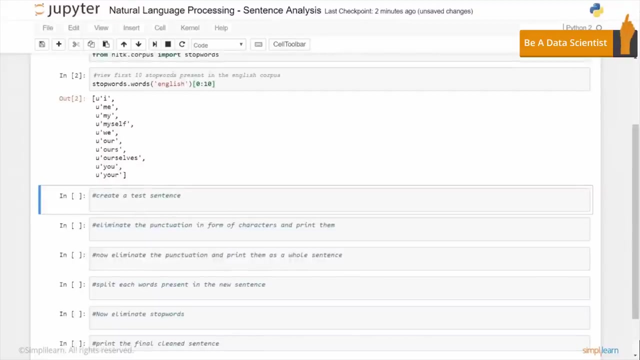 Now let's view the first 10 stopwords present in the stopwords corpus of NLTK library. This is done by passing 0 to 10 index position in the parentheses. Next let's create a test sequence to analyze. We'll create a variable testSentence and pass the sentence. 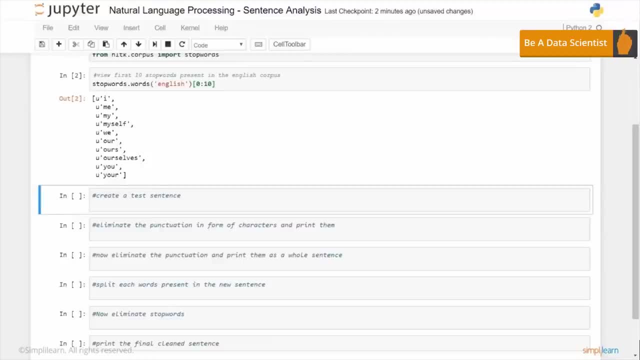 This is my first test string. Wow, We are doing just fine. First we'll use string class punctuation to remove all the punctuation present in each message, as they are also less weighted for text analysis. Then we'll remove the stopwords. 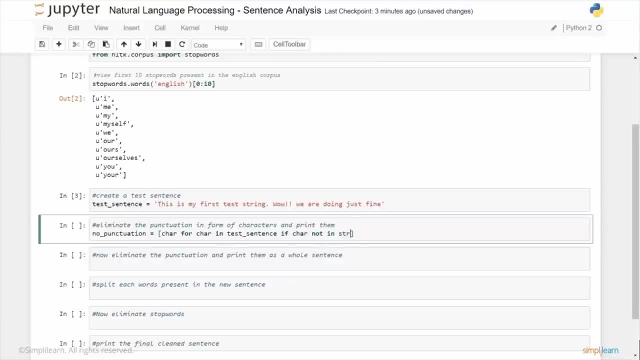 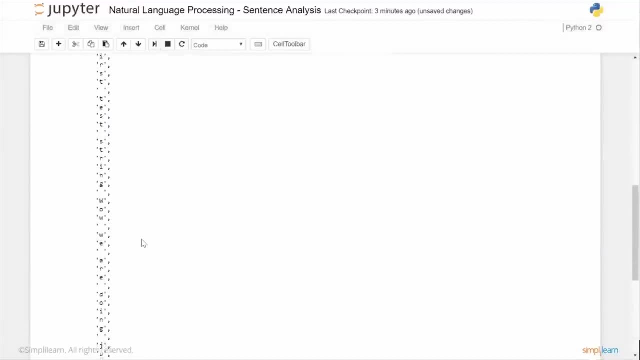 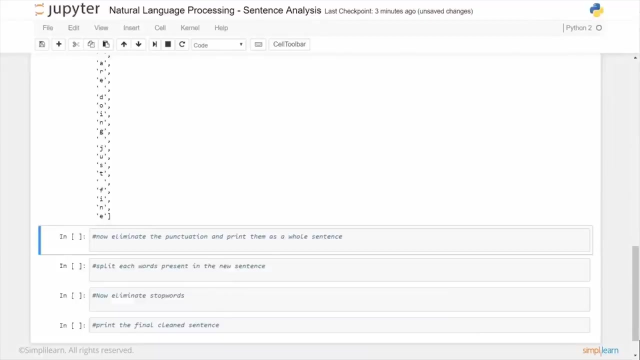 Now we'll use basic Python syntax to display the characters which don't have punctuation. As you can see, we make use of basic string class and its punctuation function. Now we'll use the stopwords corpus function to remove all the punctuation present in each sentence. 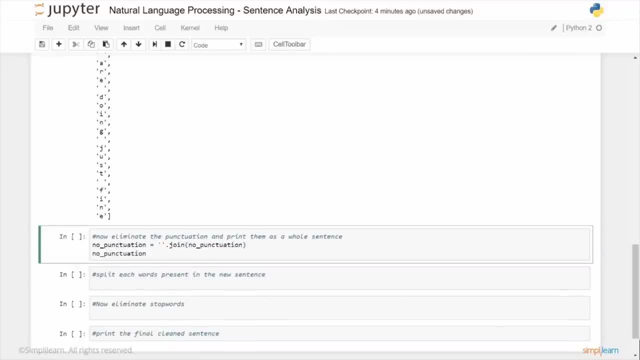 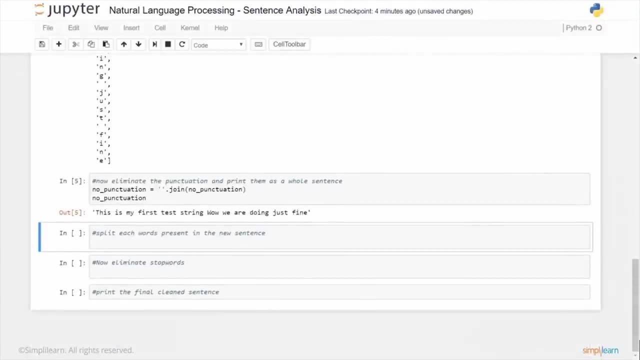 Now we'll use the stopwords corpus function to remove all the punctuation present in each sentence. We just completed the first step of the sentence analysis process. Now let's split the sentence into words. Here we can see that the list contains a lot of stopwords. 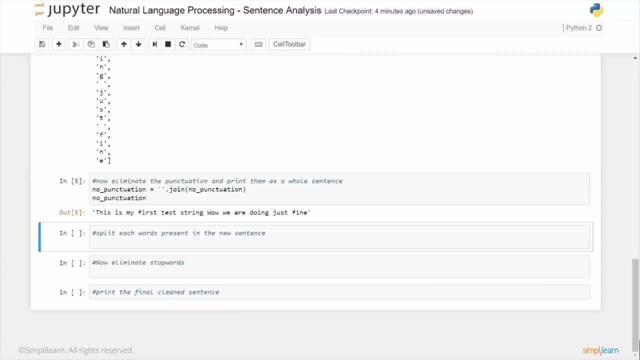 Let's remove the stopwords. We'll use stopwords, corpuswords function with English as an argument and basic Python syntax to remove all the punctuation present in each sentence and basic Python syntax. to remove all the punctuation present in each sentence. We'll use the Python word and split function to clean each word. 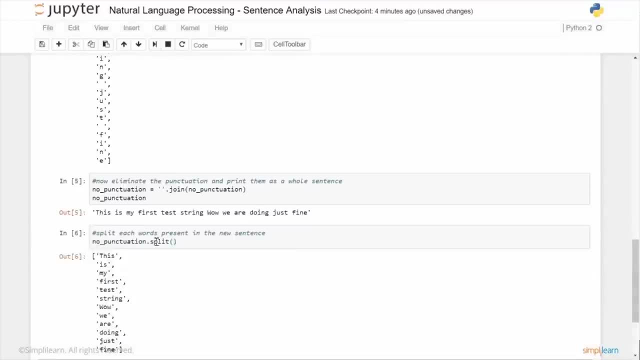 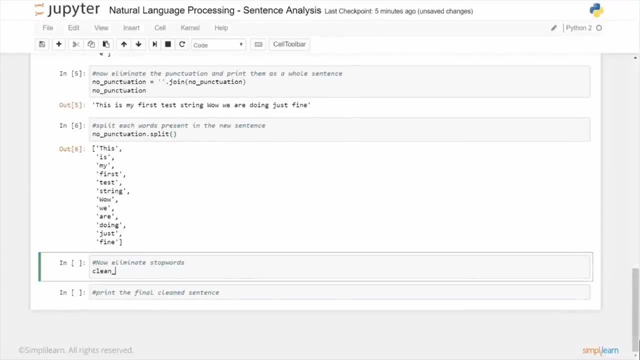 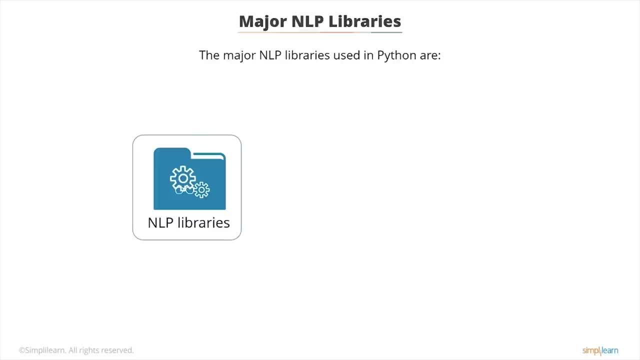 With this, we are done with sentence analysis and are sentences free of punctuation and stopwords. With this, we are done with sentence analysis and are sentences free of punctuation and stopwords. Following are the major NLP libraries used in Python. Following are the major NLP libraries used in Python. 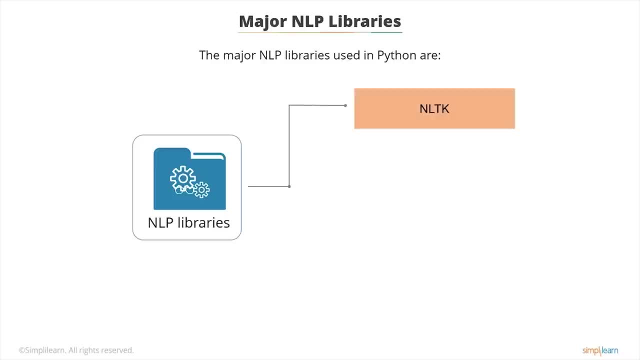 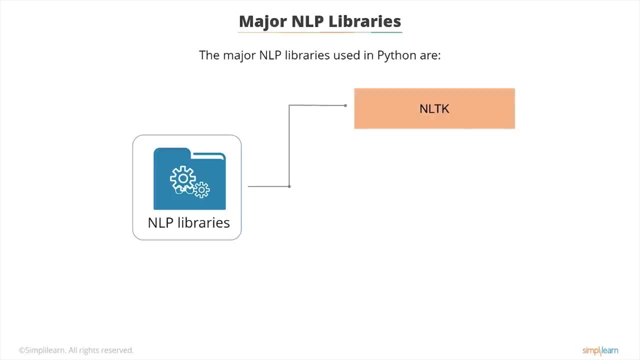 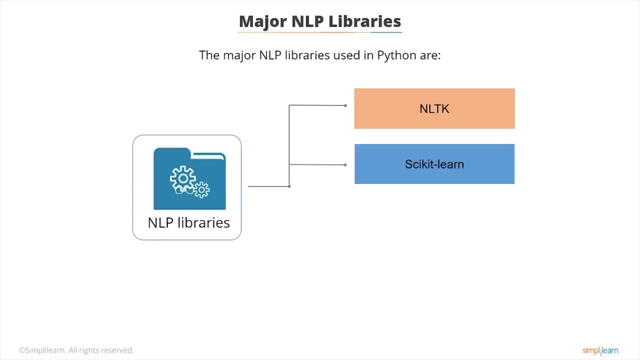 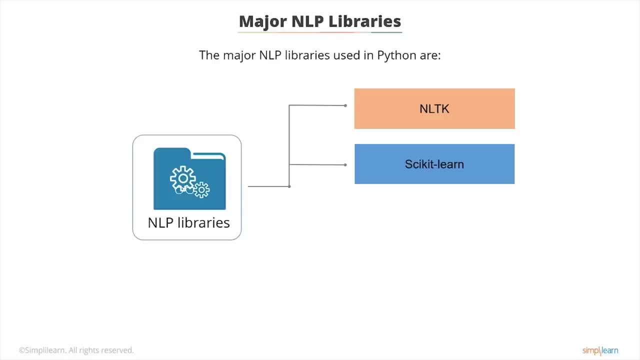 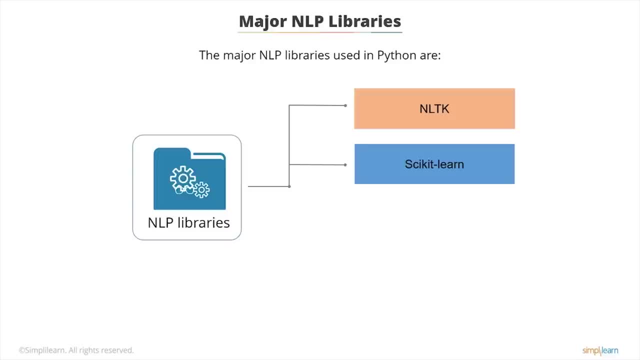 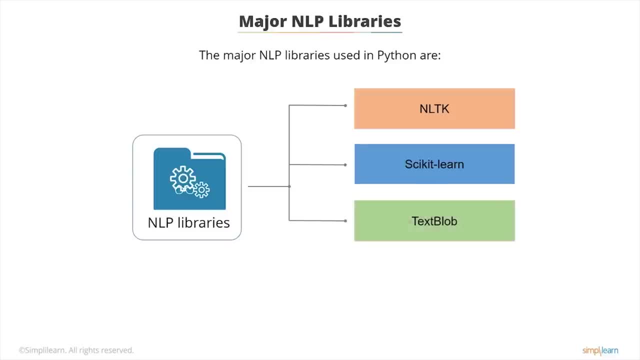 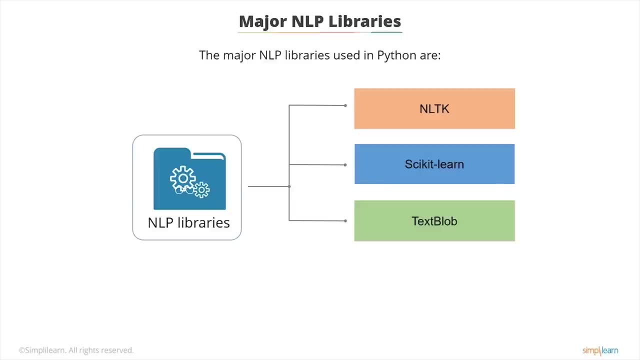 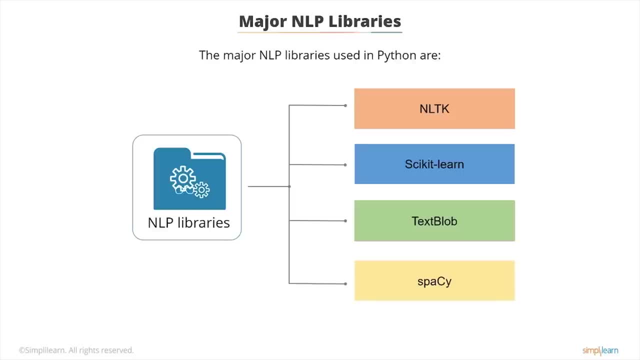 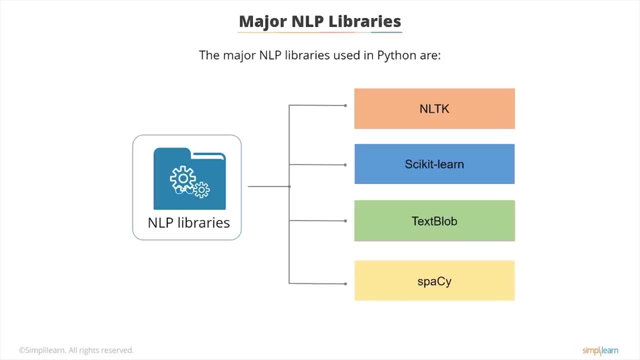 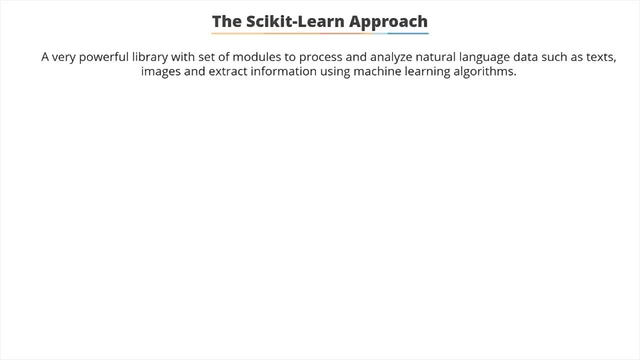 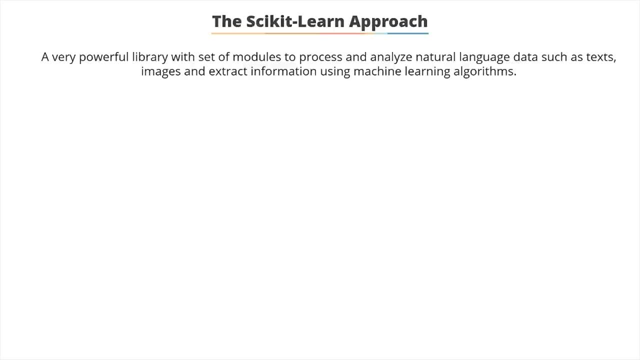 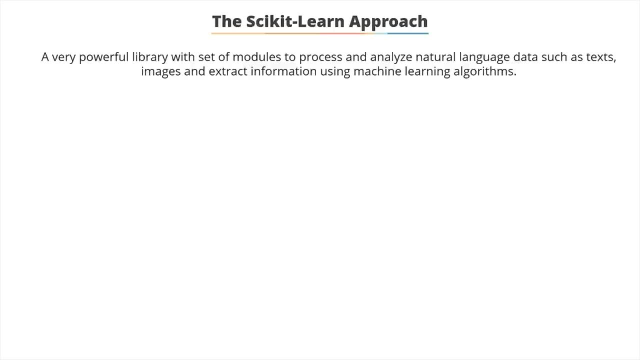 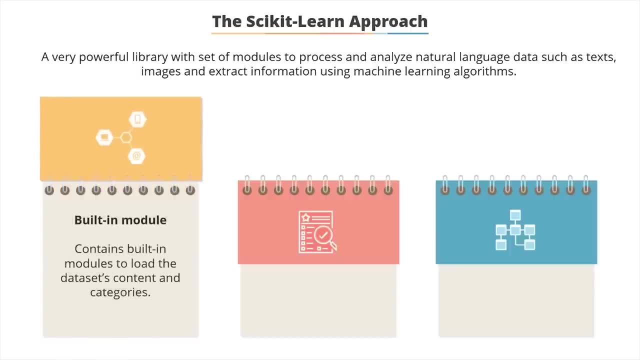 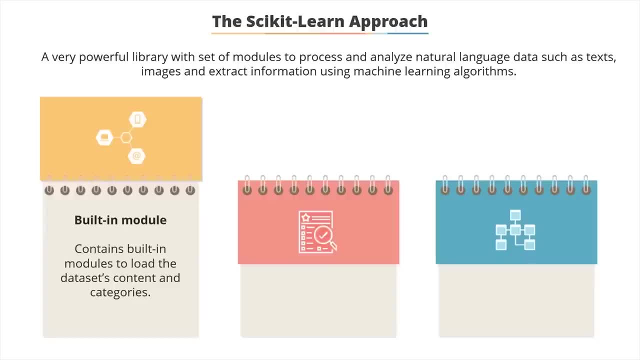 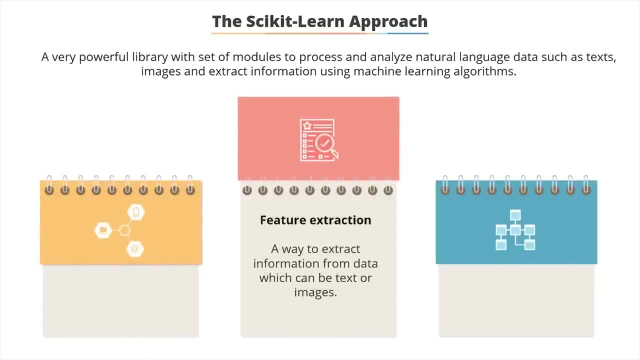 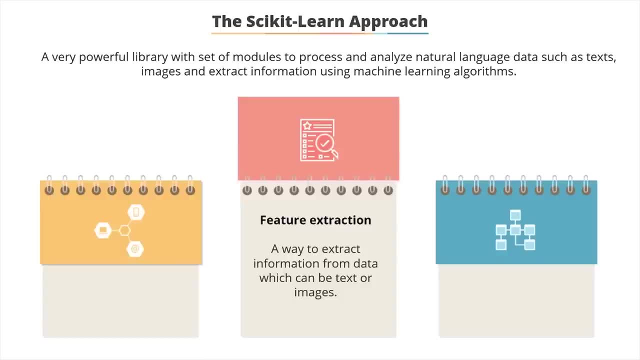 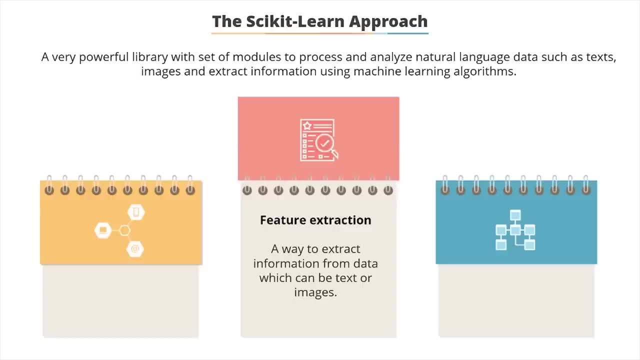 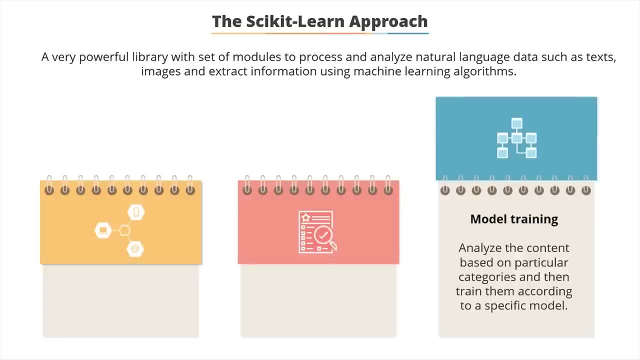 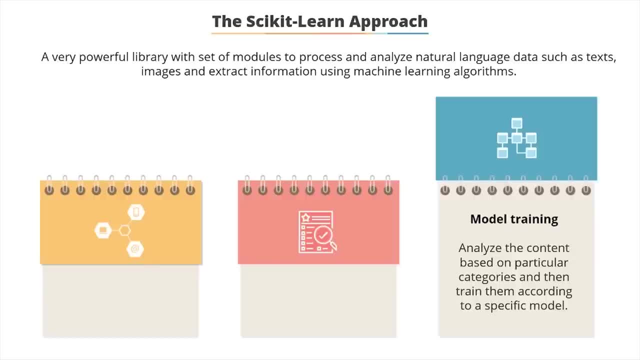 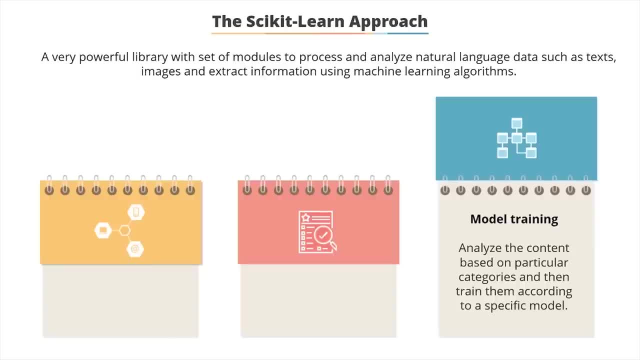 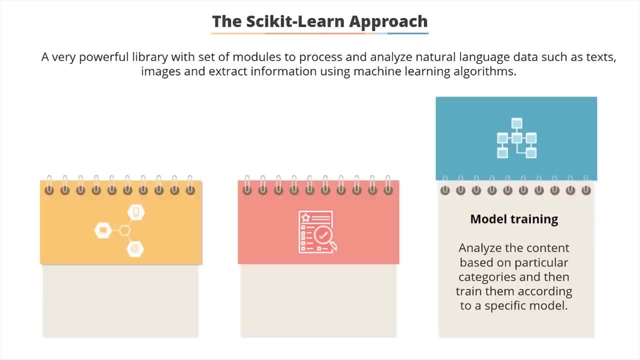 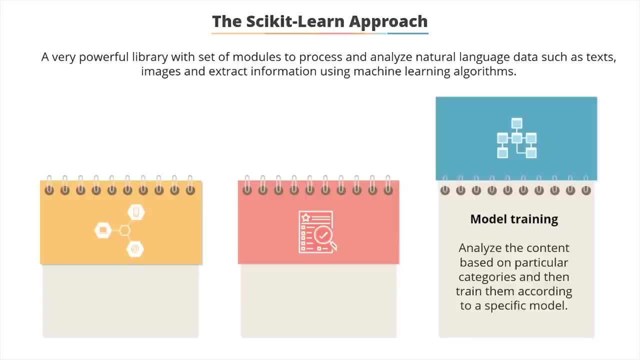 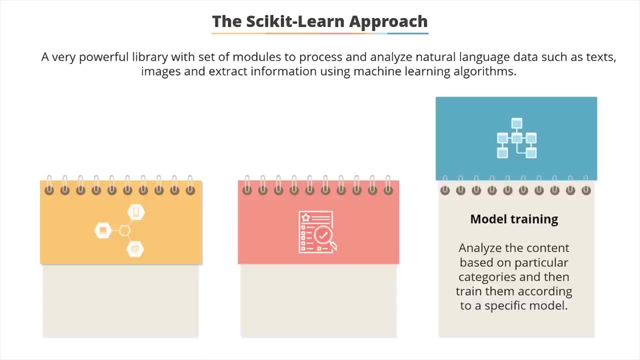 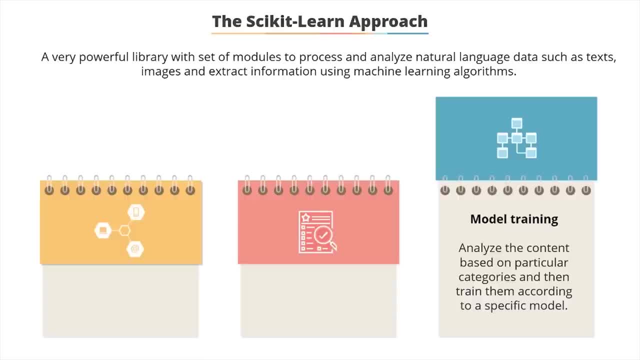 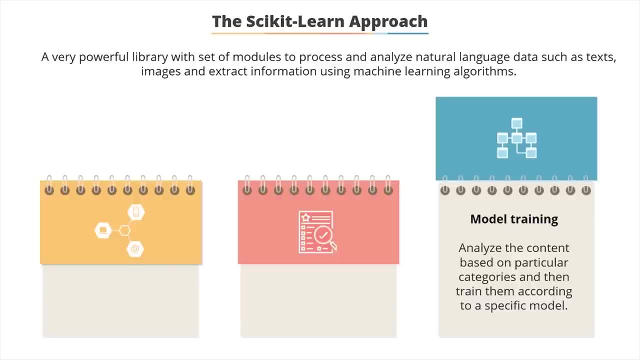 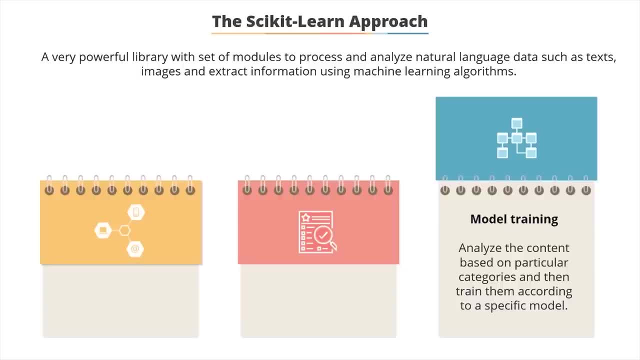 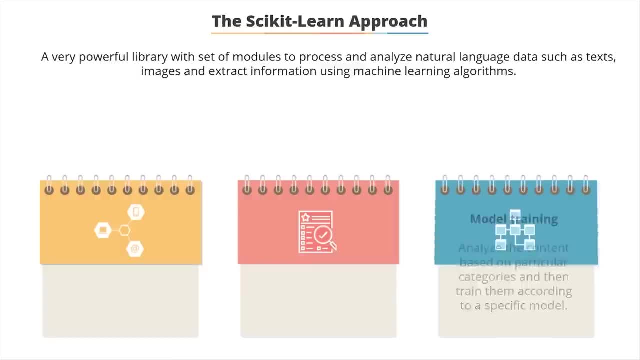 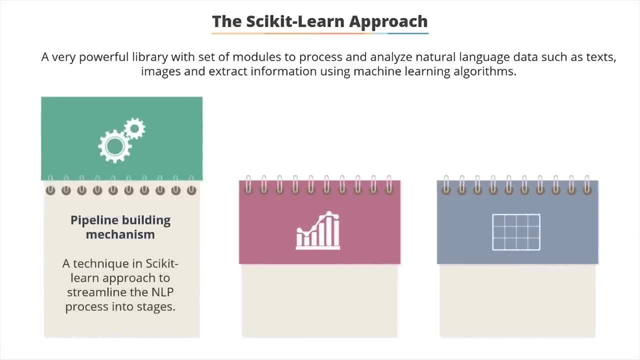 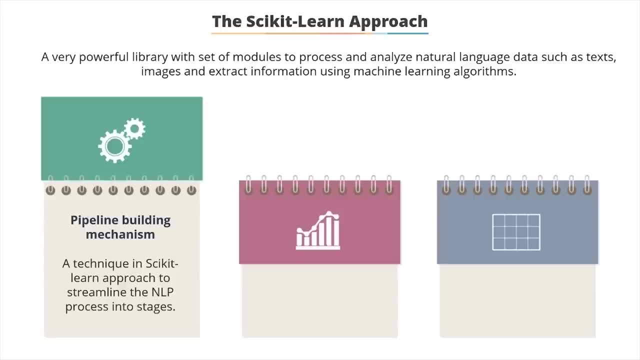 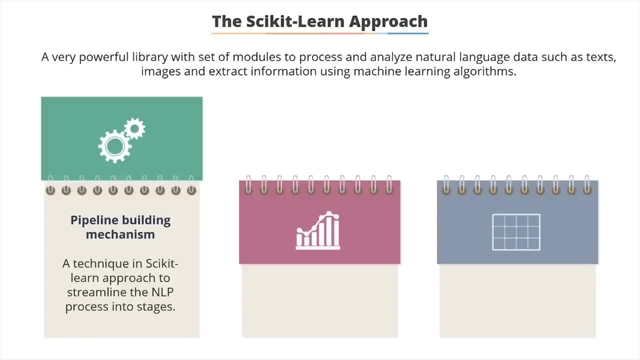 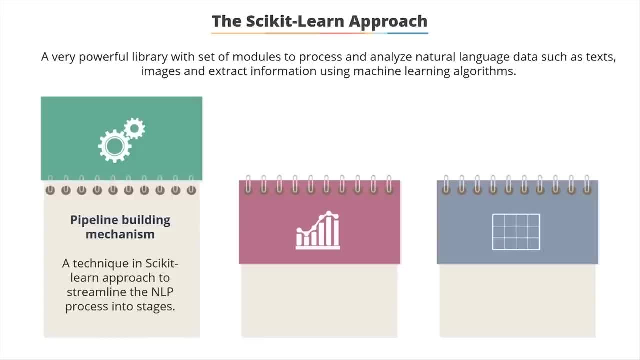 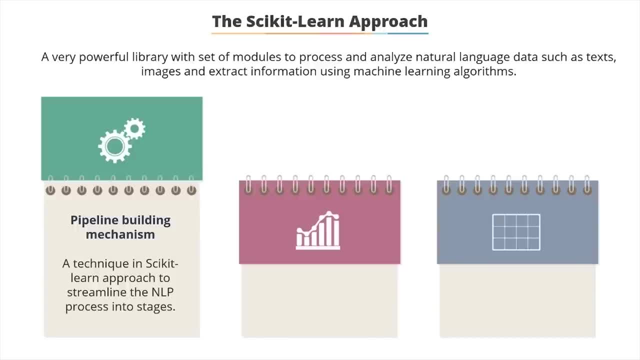 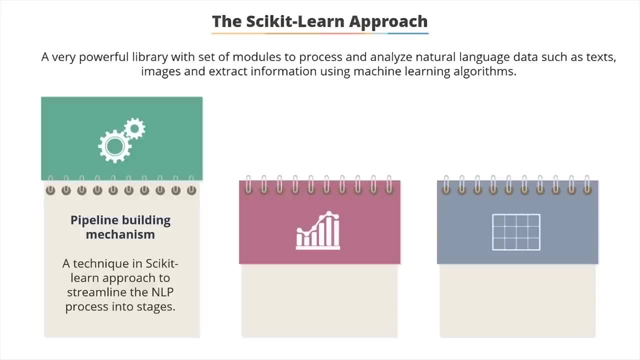 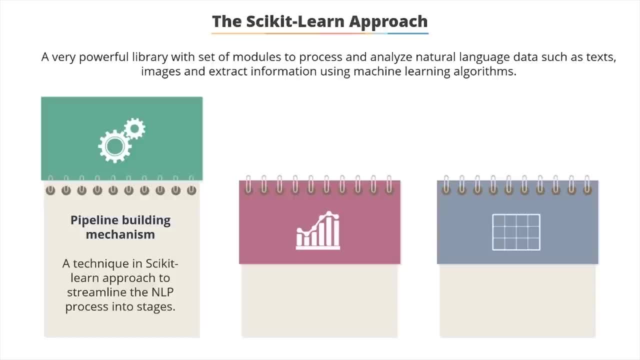 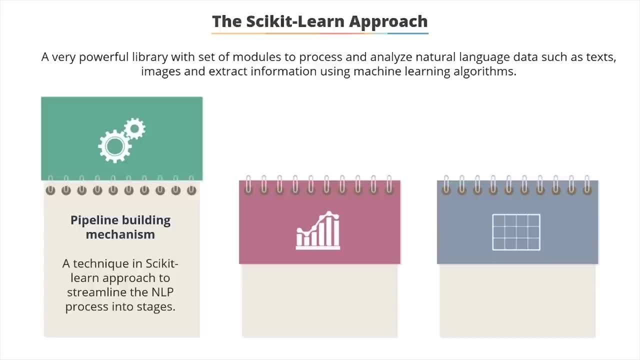 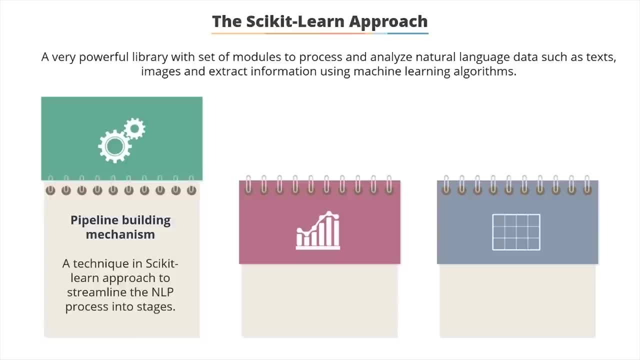 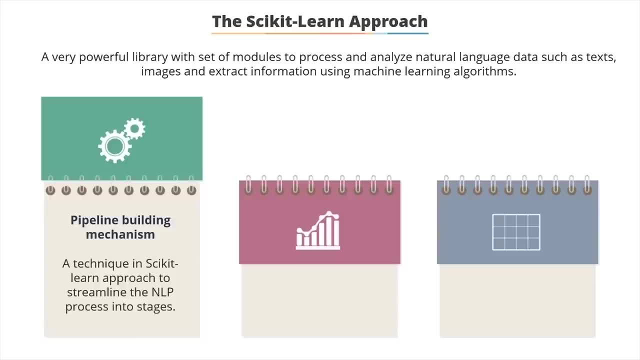 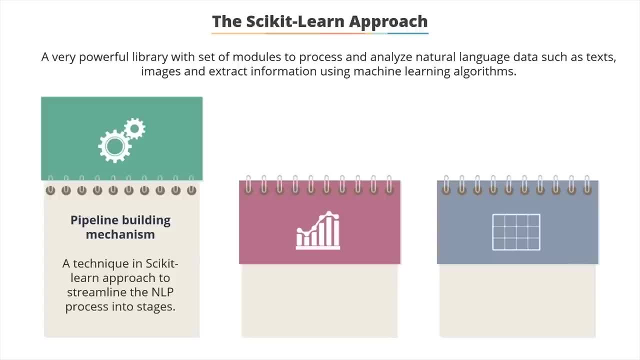 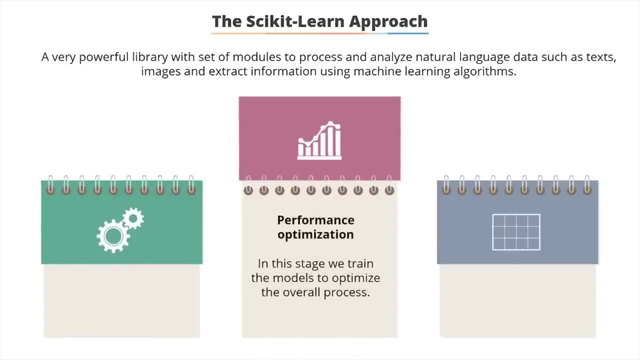 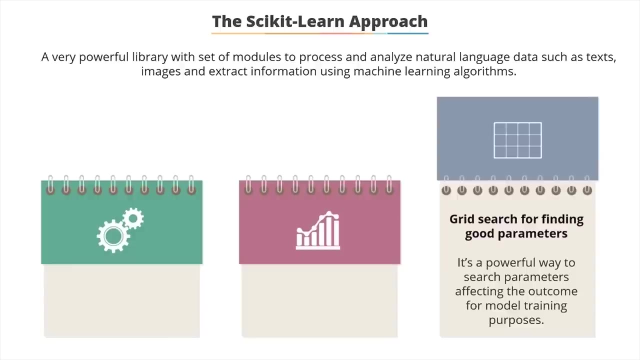 and find the sentiment analysis, Performance Optimization. In this stage we train the models to optimize the overall process. Grid Search: A model can have multiple parameters and it's a powerful way to search parameters affecting the outcome. for model training purposes, It's one of the most common ways to adjust the extracted features. 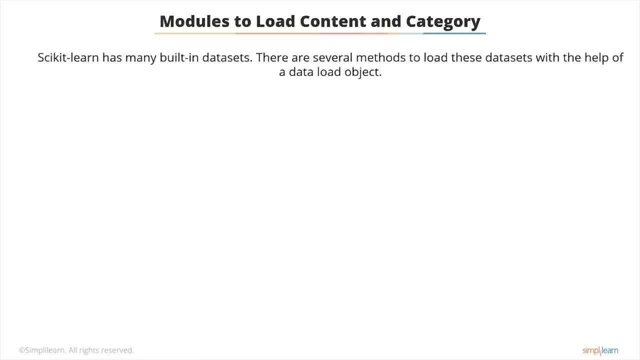 Now that you have gone through the scikit-learn approach, let's learn about its built-in modules for loading the dataset contents and categories. The diagram shows you how a dataset is loaded using methods and how the object is structured in terms of the container folder and its categories. 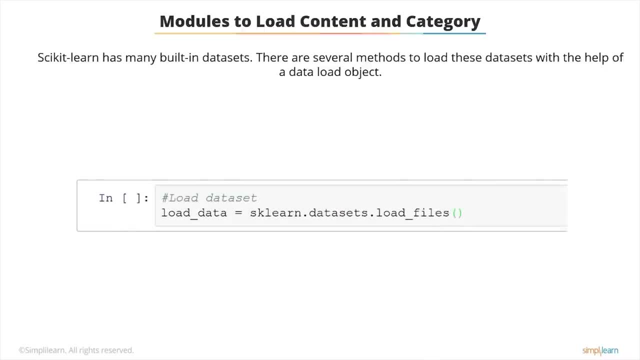 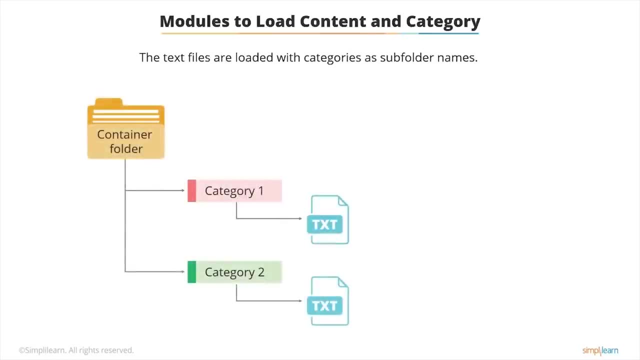 To load files you have to use the main method scikit-learndatasetsloadFiles. We can load text files with categories as subfolder names. The folder name is a folder name. Folder names are used as supervised signal label names. It doesn't try to extract features into a numpy array or scipy sparse matrix. 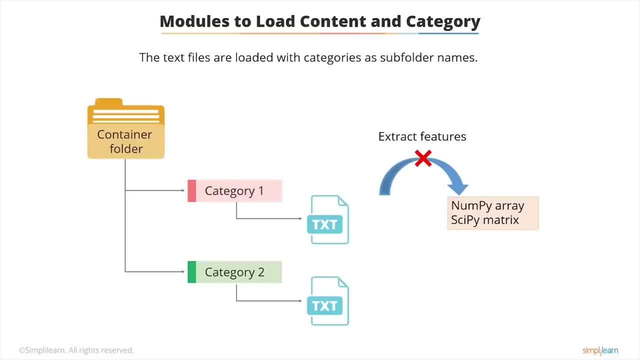 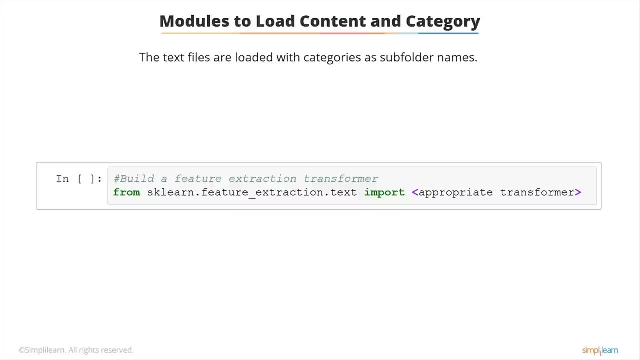 In addition, if load content parameter is false, it doesn't try to load the files in memory. To use text files in a scikit-learn classification or clustering algorithm, you'll need to use the sklearn feature extractiontext module to build a feature extraction transformer that suits your problem. 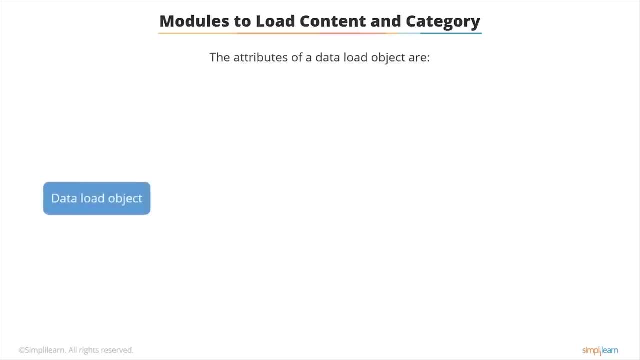 A data load object helps load the contents of a dataset. Shown here are the attributes of a data load object Bunch. It contains fields and can be accessed as dict keys or an object Target names. It's a list of requested categories. 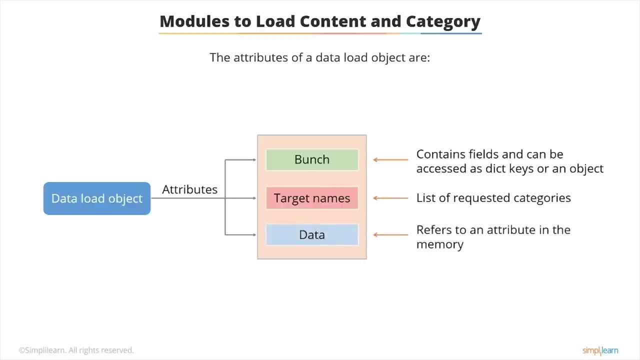 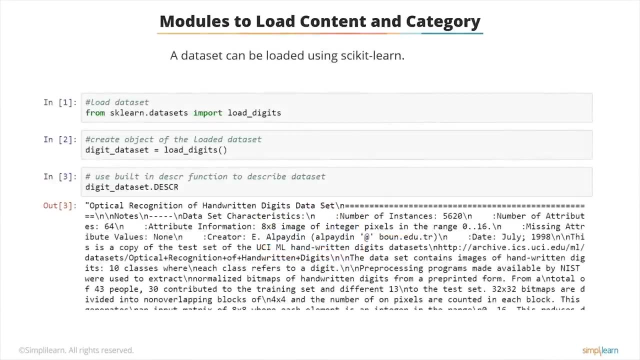 Data. It refers to an attribute in the memory where files are loaded. Let's see how a dataset can be loaded using scikit-learndatasetsloadFiles. There are several datasets that can be loaded. Let's load the digits dataset to view the data using built-in methods. 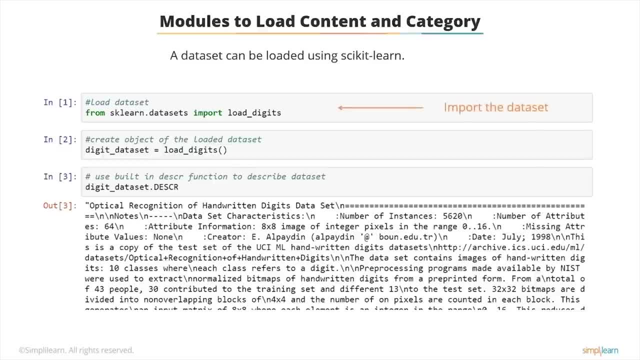 Perform the following steps: 1. Import the desired dataset: Use the syntax from sklearndatasetsimportLoadDigits. 2. Load the dataset by creating an object, As we had discussed earlier. a data load object is used to load contents. 3. Describe the dataset using DESCR function. 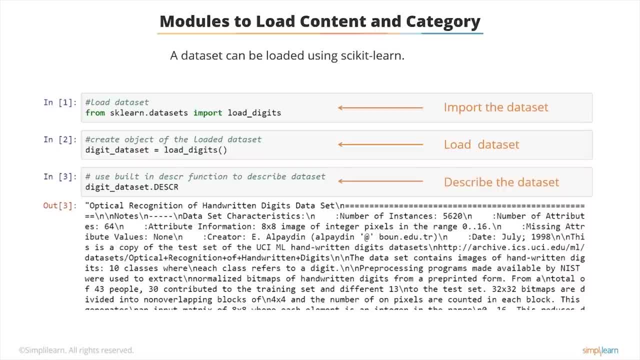 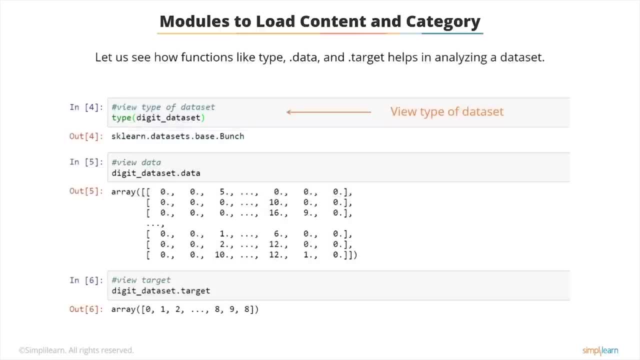 Using this function, you can view all of the information which describes the dataset. Next, let's view the dataset type. Use the syntax type digitsDataset. As we can see, the type of the dataset is Bunch. To view the data of the digits dataset, apply the function data. 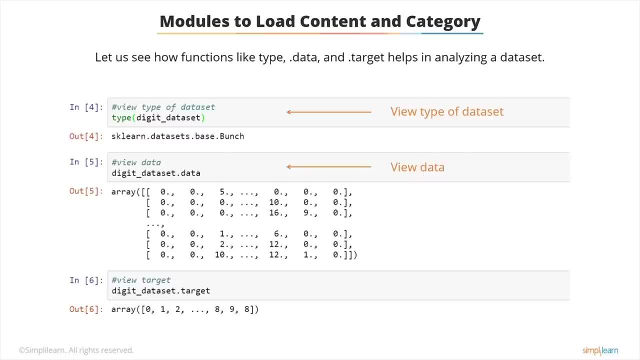 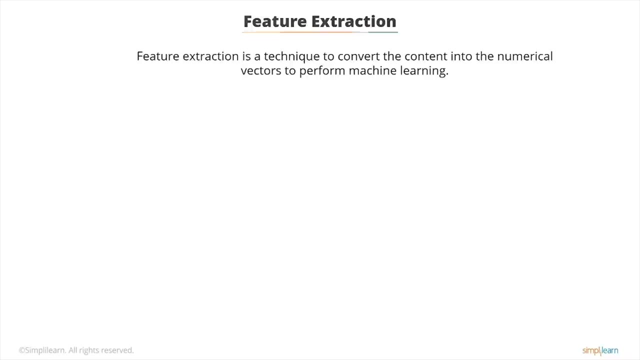 The output displays the actual data which is bound to the dataset. Let's view the target with the function target. The arrays displayed here are the response data which is present in the dataset. Next, let's talk about feature extraction, another functionality of the scikit-learn approach. 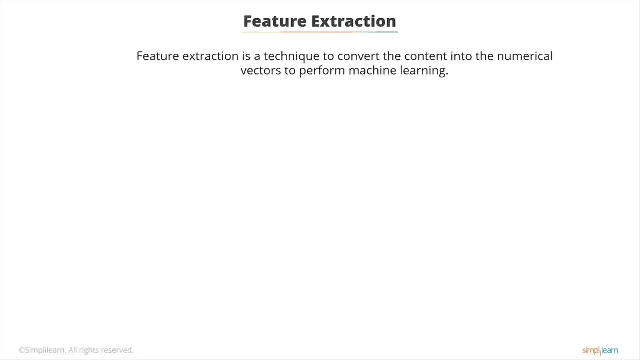 This is a technique to convert the content into numerical vectors to perform machine learning. The feature extraction technique is used mostly in machine learning while dealing with text or image data. There are two major types of feature extraction techniques: Text feature extraction: It's used to extract features from text data. 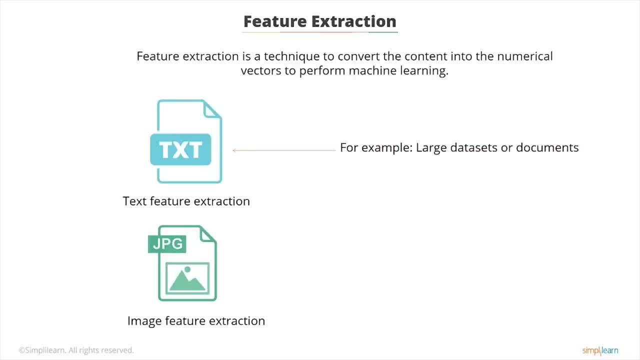 Examples include large datasets or documents. Image feature extraction: It's used to extract image features. Examples include patch extraction or connectivity graph of an image forming contiguous patches, also known as hierarchical clustering, Bag of words. Now let's learn about the bag of words. 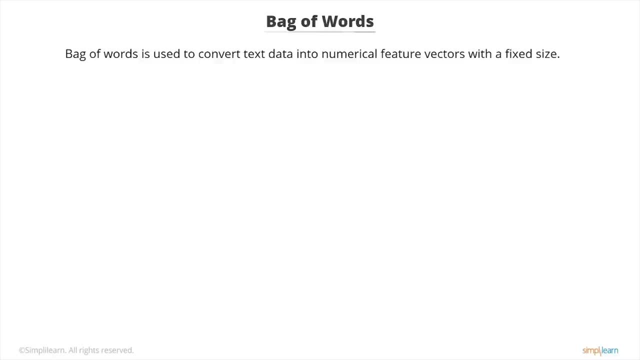 which is one of the most common text feature extraction techniques. It's used to convert text data into numerical feature vectors with a fixed size. Let's see how it works by considering a document where we need to extract text features. The steps to follow are: 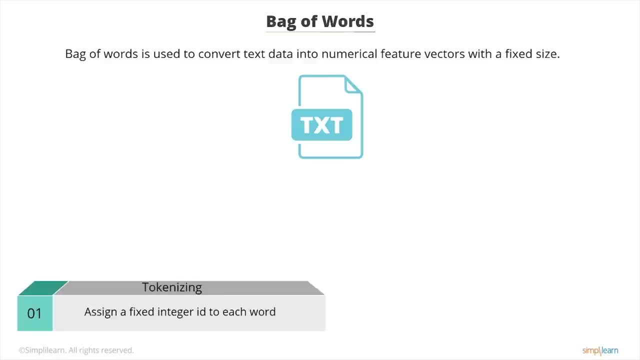 Assign a fixed integer ID to each word by splitting them into several words, also known as tokenizing. Then count the number of occurrences of each word or token. Finally, store it as the value feature in matrix format. The matrix presentation on the screen shows how multiple documents and tokens are structured. 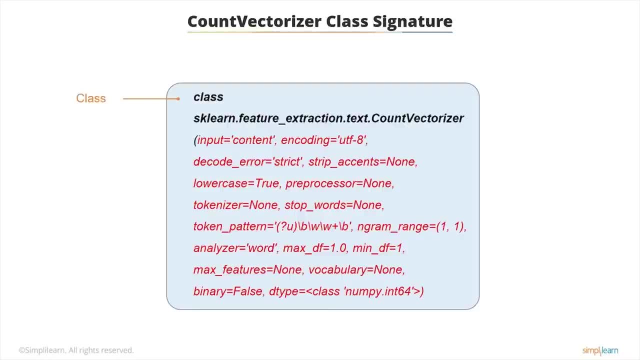 This screen shows how the count vectorizer algorithm works in Scikit-Learn. The goal is to convert a collection of text documents to a matrix of token counts. There are several parameters which affect the vectorization process. Let's take a look at the components of the signature. 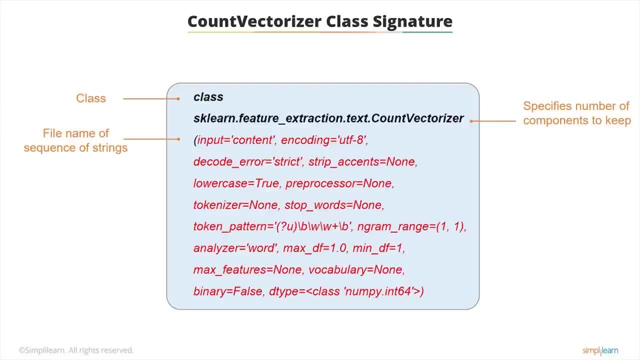 Input content. The input content can be a file name of the sequence of strings which needs to be vectorized Encoding. The default encoding is UTF-8.. The encoding is to decode the input Strip accents: It removes accent present in the code. 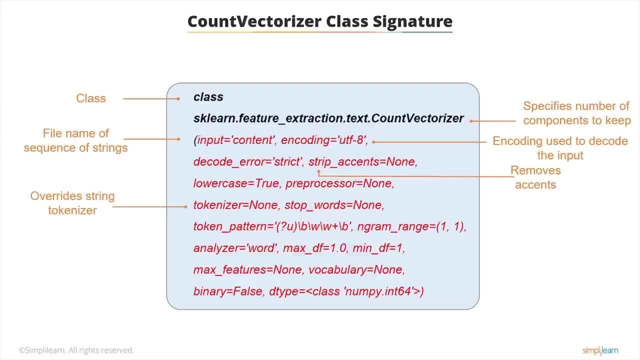 Tokenizer: It overrides the string tokenizer method, but the default value is none. Stop words: It's a built-in stop words list that is used. Max threshold: It indicates the terms or words that appear more than a given threshold value and should therefore be ignored. 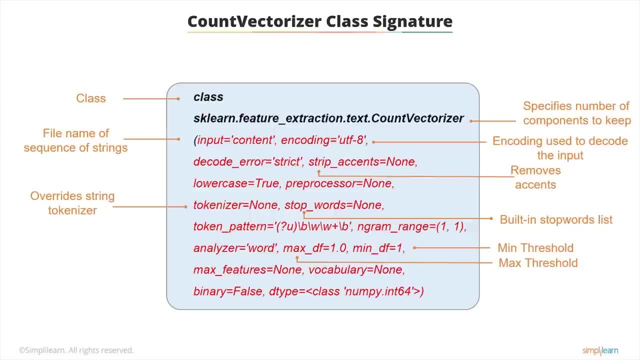 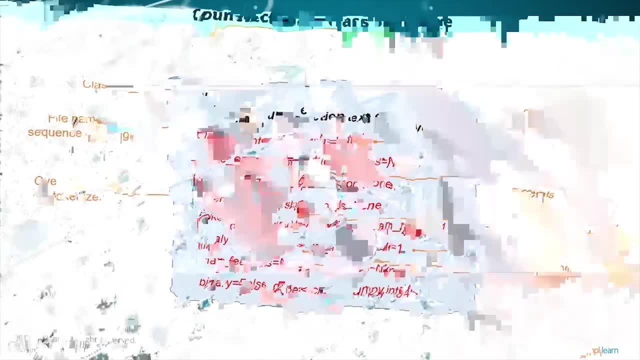 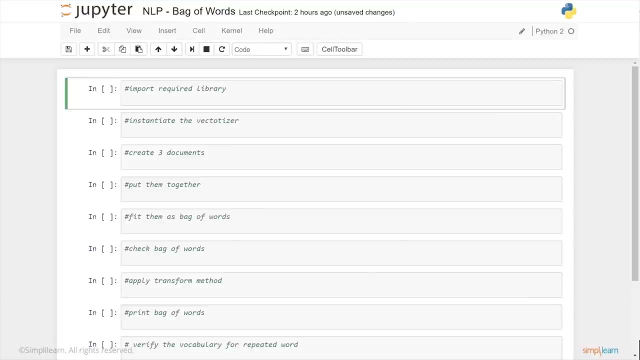 Min threshold. It indicates the terms or words that appear less than a given threshold value and should therefore be ignored. In this demo, you'll learn how to process documents Using Bag of Words. Let's start by importing the required library. 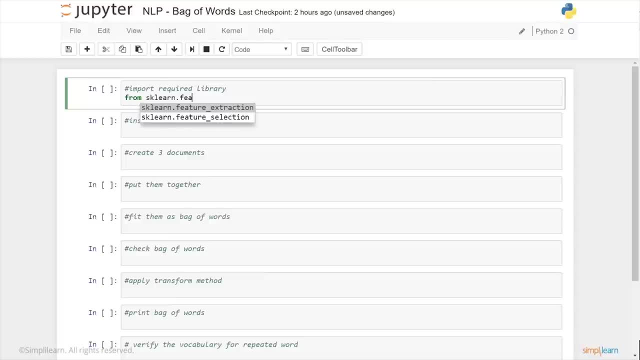 CountVectorizer class. This class helps tokenize the document. It converts the text into vectors by assigning numeric values to each word. Let's create an object vectorizer by instantiating the CountVectorizer class. Next, we'll create three random documents. Let's add some text to the documents. 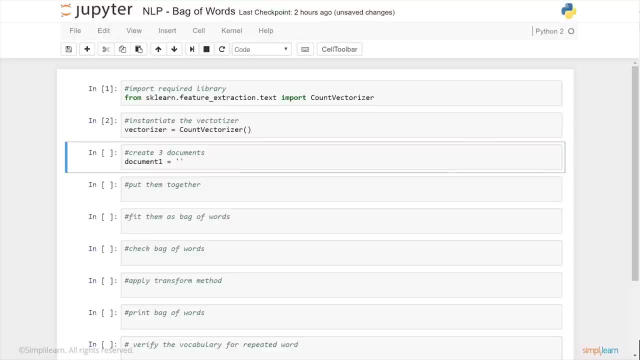 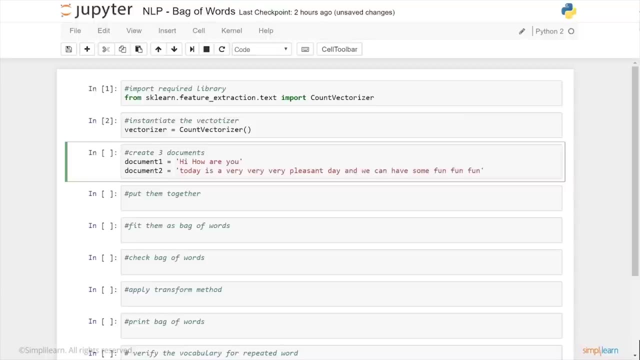 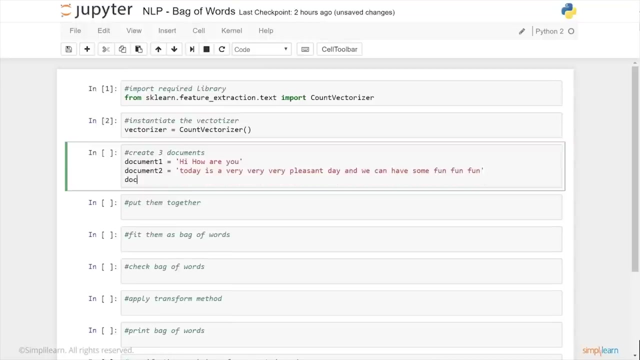 Document 1 can have: Hi, how are you? In Document 2, we can add: Today is a very, very, very pleasant day and we can have some fun, fun, fun. And in Document 3, we can say: 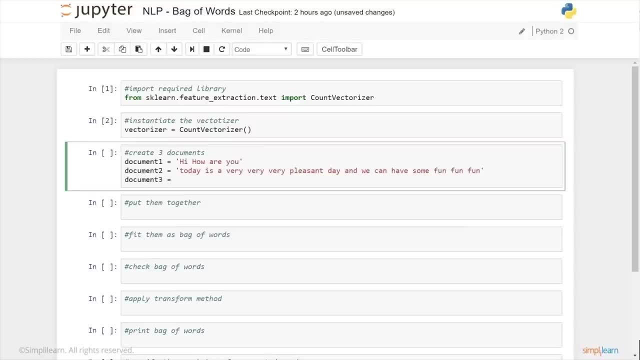 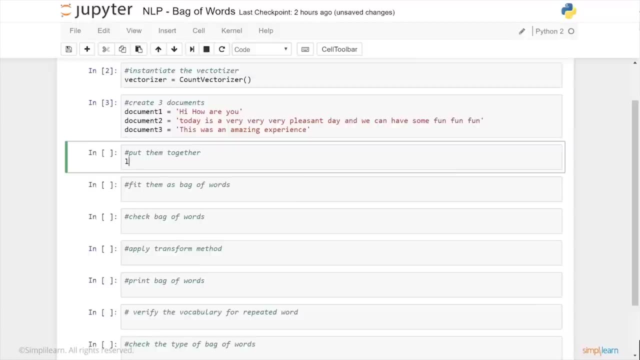 This was an amazing experience. This was an amazing experience. Now put all three documents together as a list. Next comes the interesting part, which is creating the Bag of Words for the list of documents. This is done by accessing the fit method and fitting the documents into the vectorized object. 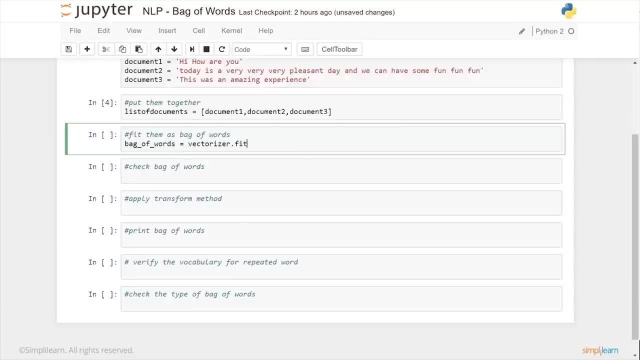 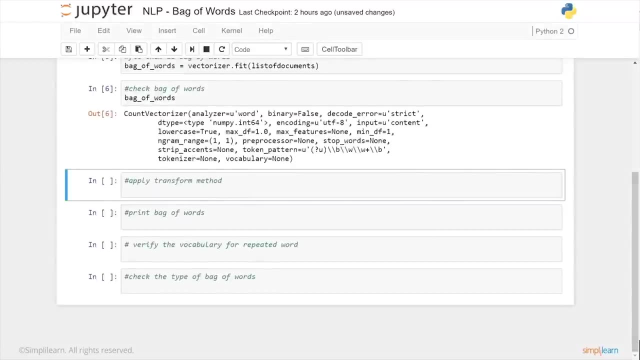 We'll move on to accessing the transform method and transform the list of documents. We'll move on to accessing the transform method and transform the list of documents. Now let's print the Bag of Words and look at the details. You can see the properties of vectorized object. 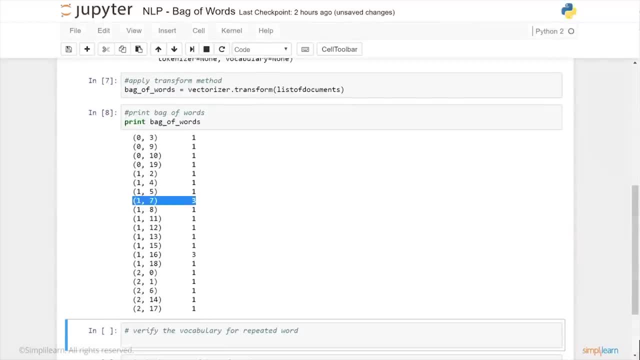 As you can see, the first number is the tuple and the second number is the frequency of words. The tuple here indicates the document number and feature indices of each word which belongs to the document. Feature indices are generated from the transform method. This is a feature extraction process. 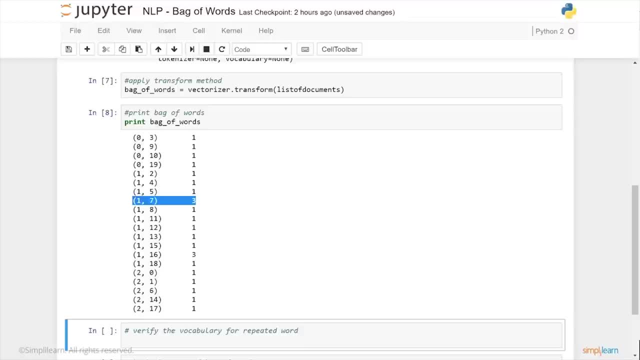 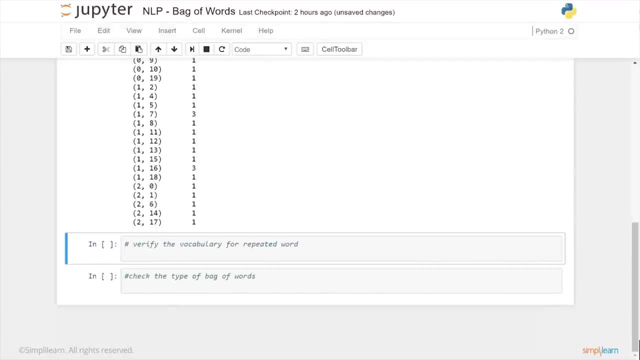 and to extract the features, you have to refer to the indexes which is assigned to any particular feature. Next, let's check for repeated words in the vocabulary that is built with the get function and then print it. Finally, check the Bag of Words type for the documents. 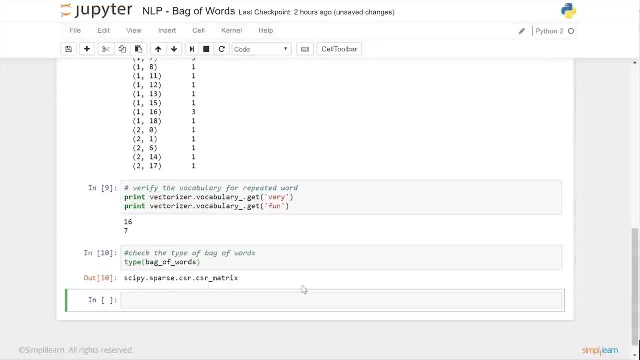 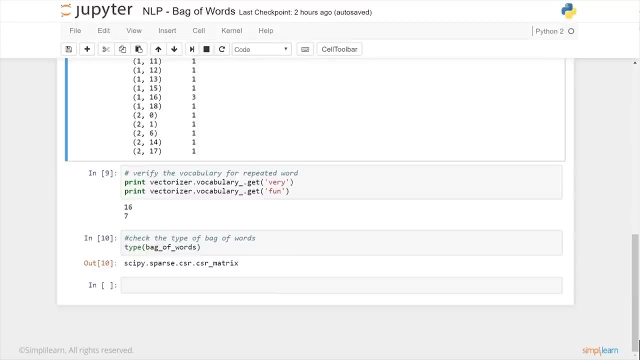 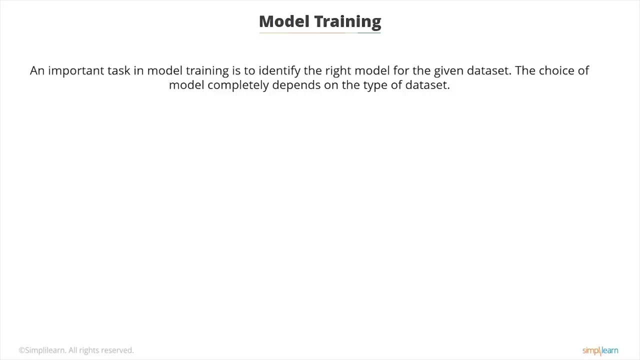 Finally, check the Bag of Words type for the documents. The output displays sparse matrix and it falls under SciPy. In this demo, you learned how to use Bag of Words technique and transformed documents using the transform method. The next feature of Scikit-learn is model training. 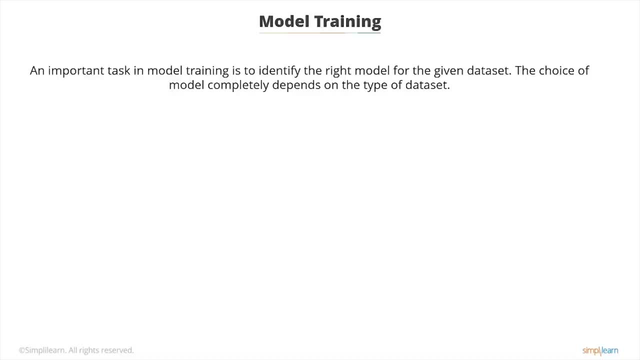 An important task in model training is to identify the right model for the given dataset. Scikit-learn provides a range of models to choose from and also trains them by using the extracted features from the dataset. The choice of model completely depends on the type of dataset. 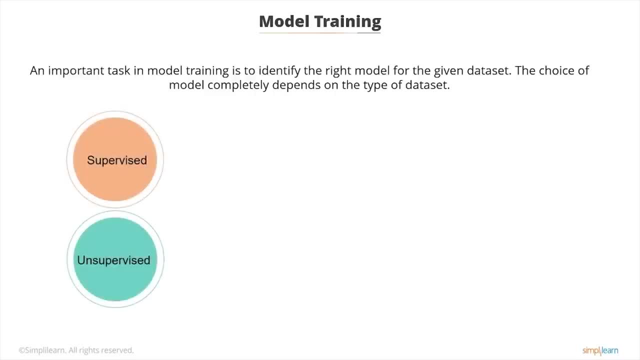 The models can be trained as a supervised learning model or unsupervised learning model. Supervised learning model: For a given dataset, we'll have observations, features and response. In supervised learning, we make use of all three tasks: predict the outcome of new observations and datasets. 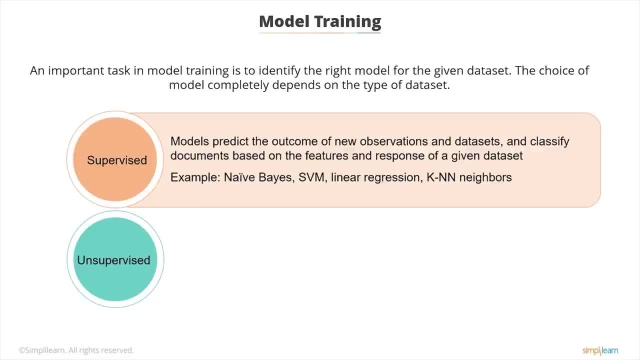 understand which predictors affect the response or outcome and generalize the data and find the right answer. Generalization is also known as making predictions. Models can be trained to classify the documents based on the features and response, For example, naive Bayes, SVM, linear regression and KNN neighbors. 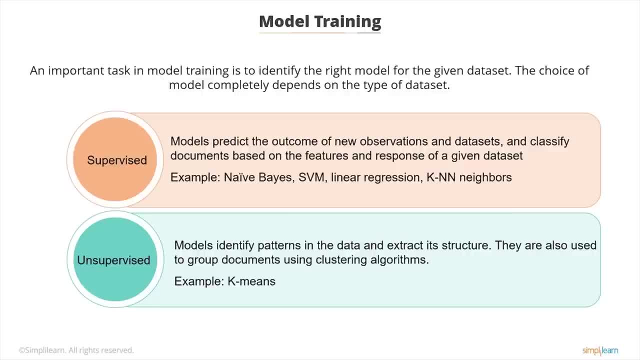 Unsupervised learning model. In this type of learning the response or the outcome of the label of the data is not known. There is no definite or right answer in this model. So here we try to train the model by following a few steps. 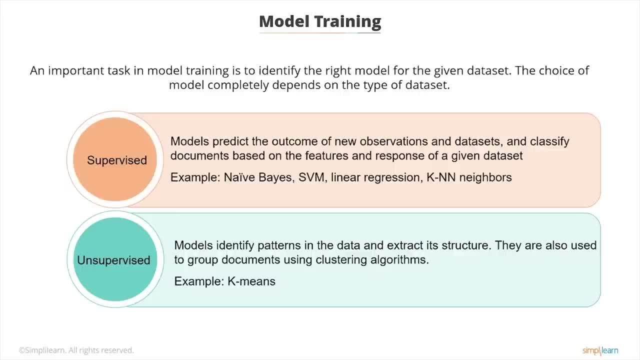 such as understanding the structure of the data first and identify the pattern in the data finding predictors that behave in the same fashion or have some familiarity, exploring the dataset and the goal as representation of the data. Representation is also known as extracting structure. Unsupervised model can also be used to group documents by applying clustering algorithms. 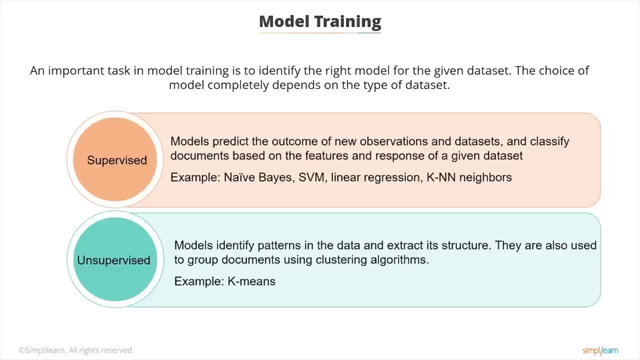 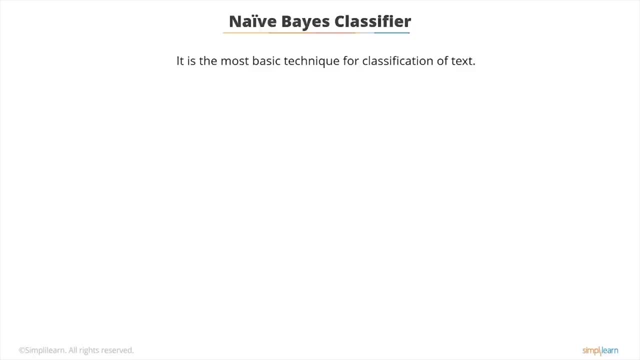 For example, clustering text documents using K-means. Naive Bayes is a basic technique for classification of text. It assumes that the probability of each attribute belongs to a given class value and is independent of all other attributes. The advantages of Naive Bayes classifier. 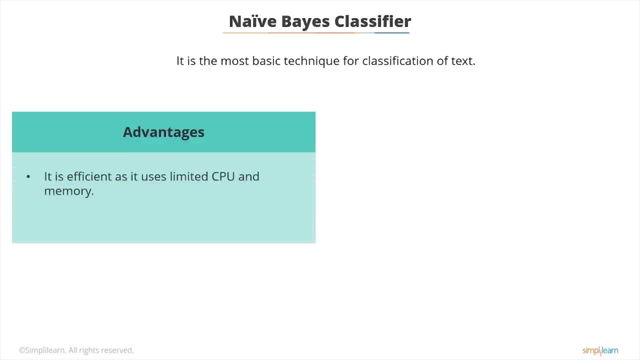 It performs the task with limited CPU and memory, Therefore it's very efficient. It's fast, as the model, training time is very less. Naive Bayes is heavily used in sentiment analysis, email spam detection, categorization of documents and language detection. 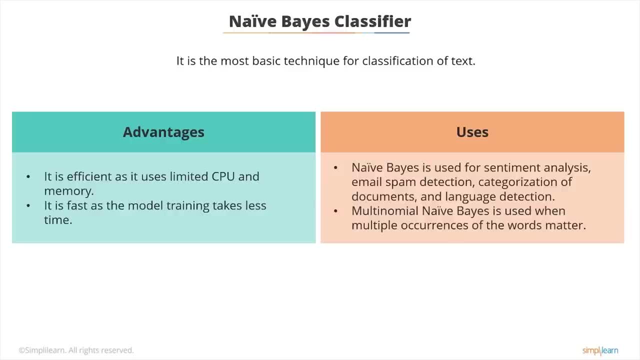 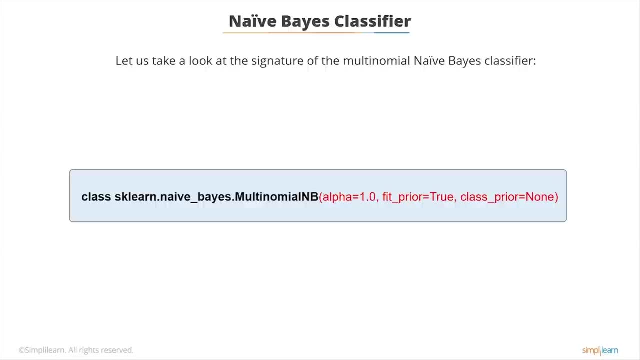 Multinominal Naive Bayes is used when multiple occurrences of the words matter. Multinominal distribution normally requires integer feature counts. Let's take a quick look at the Scikit Multinominal NB model class. There are three major parameters in this class. 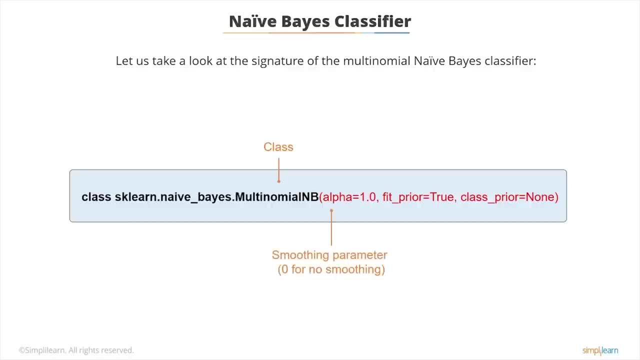 Alpha. It's also known as Lap Place Transform or smoothing parameter, and is mainly used for categorical data. Fit Prior. It indicates whether to learn class prior probabilities or not. If false, a uniform prior will be used. But, as you noticed, the default is true. 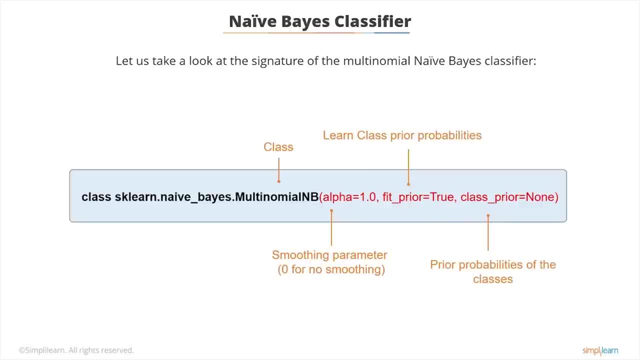 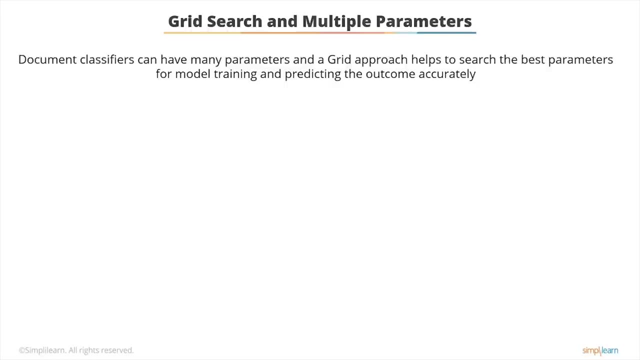 Class Prior. The default is none but if specified, the prior class is adjusted according to the data. The next feature of Scikit Learn we'll be looking into is Grid Search. We use a document classifier to predict the category of a document. 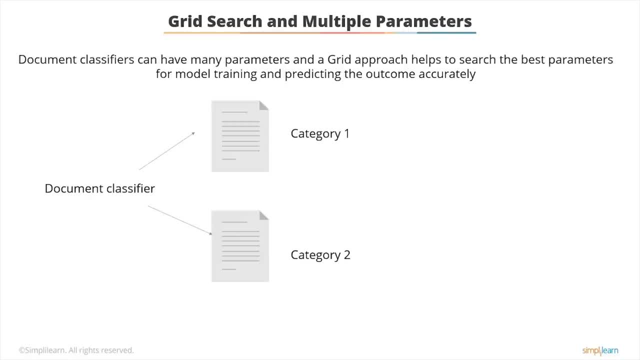 To try predicting the outcome of a new document, we need to extract the features. A document classifier can have many parameters and a grid approach helps to search the best parameters for model training and predicting the outcome accurately. When we create a model, it ends up with multiple parameters. 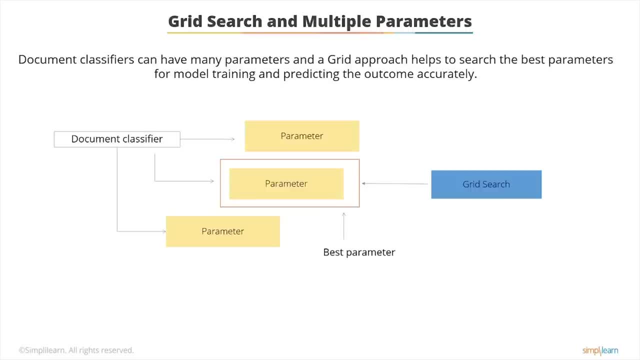 It would be too tedious to run through each parameter and tweak it. In such cases, a grid search is useful. The whole dataset can be divided into multiple grids, like a chessboard, and the search can be run on entire grids or a selected combination of grids. 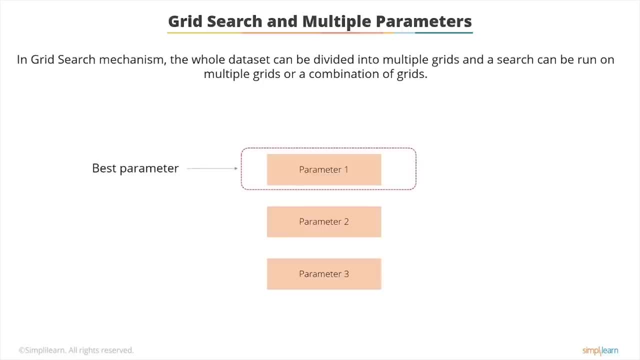 So we use a grid search mechanism to perform an exhaustive search on the best parameters which affect the model. However, this approach has some constraint, such as the whole grid search process is subjected to availability of the CPU cores of the system. This is owing to the fact 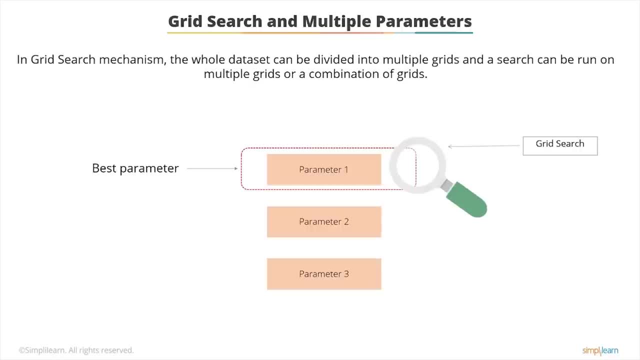 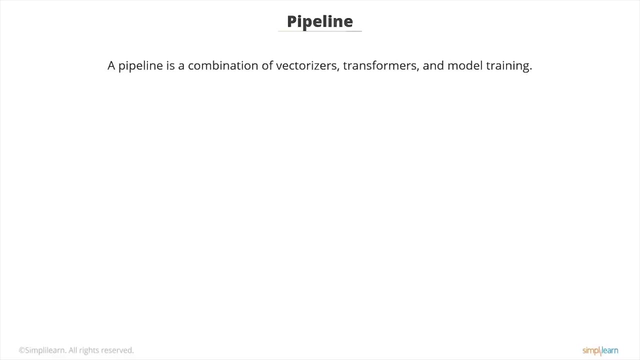 that there can be several parameters and running an exhaustive search can impact the system performance by taking more of the CPU memory. So far we have learned that there are three major steps for analyzing text data: 1. Vectorizer: This is a general process. 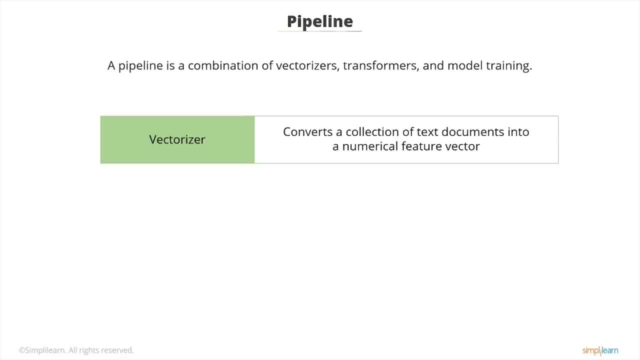 of converting a collection of text documents into a numerical feature vector. In vectorization, the documents are split into words or tokens, and each document is assigned a number 2. Transformer. During transformation, you find the occurrence of each word in a document. 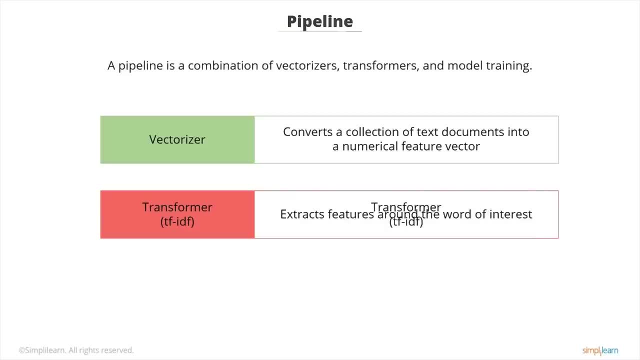 This process is primarily used for feature extraction. 3. Classifier or model training. This is required for accurate predictions. A model uses training and testing datasets to optimize its overall performance. For example, different algorithms are used to classify text documents and find the sentiment analysis. 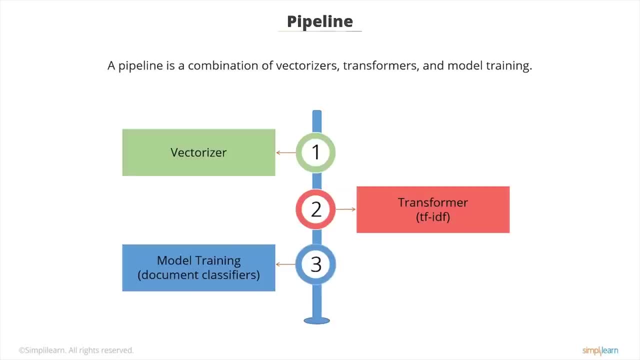 This is where Scikit-learn becomes more productive by creating the pipeline for the dataset. A pipeline is essentially a combination of these three steps, So using Scikit-learn, pipeline can be created and we can train the model using a single command. 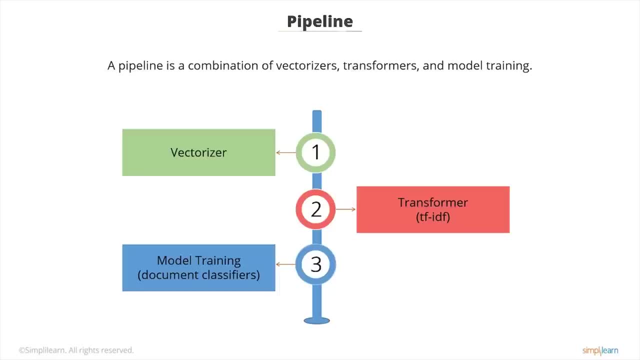 We just need to put them all together in a single class and create a pipeline to operate on a given dataset. The main purpose of the pipeline is to assemble several steps that can be cross-validated while setting different parameters. 4. Processing In this demo. 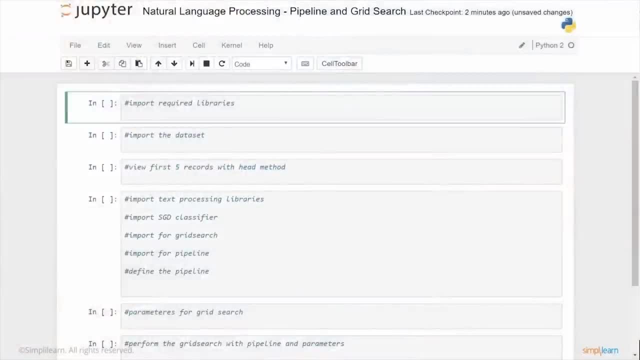 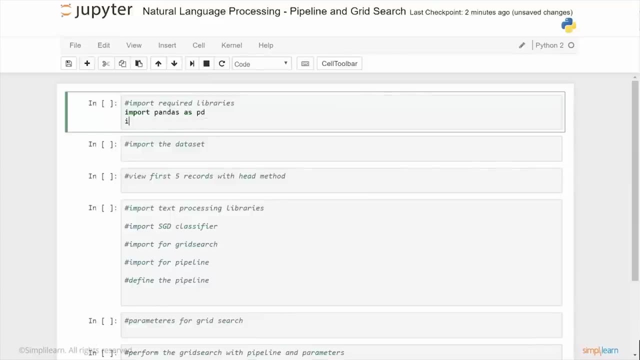 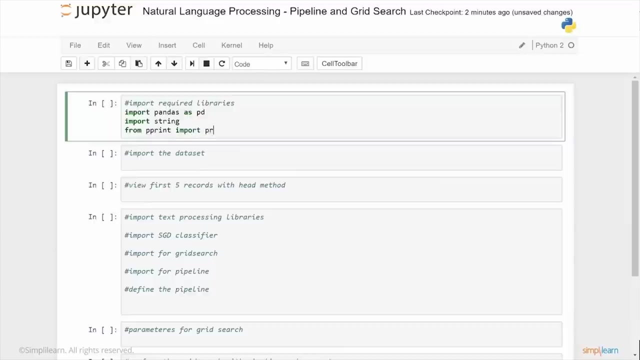 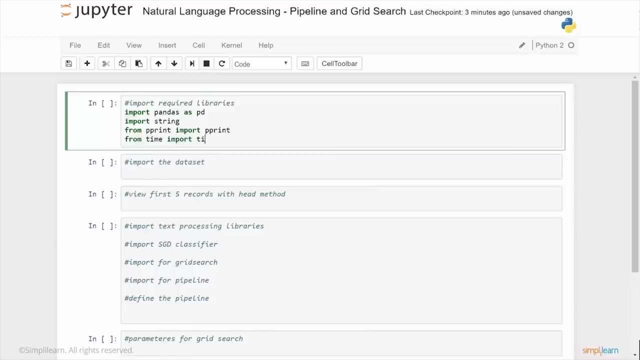 we'll learn how to apply pipeline and grid search. Let's start by importing the required library: pandas string, print and time. Next we'll get the spam data collection with the help of the pandas library. Here the backslash t indicates: 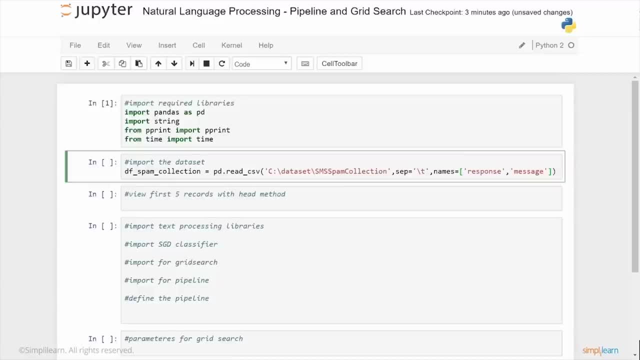 that data in the spam dataset is tab-separated or tab-delimited, and set function takes it as a parameter. Also, message is a feature which refers to the text present in the dataset. Response is the label or the category of the message. Let's view the first five records. 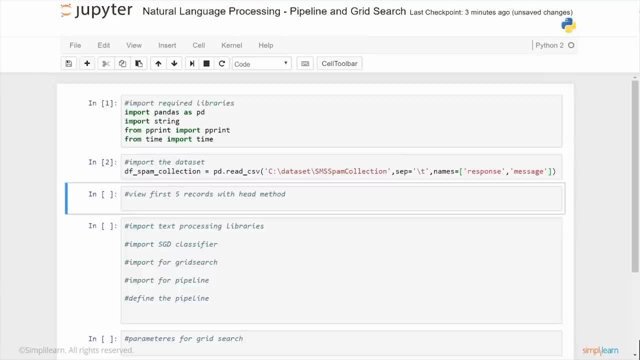 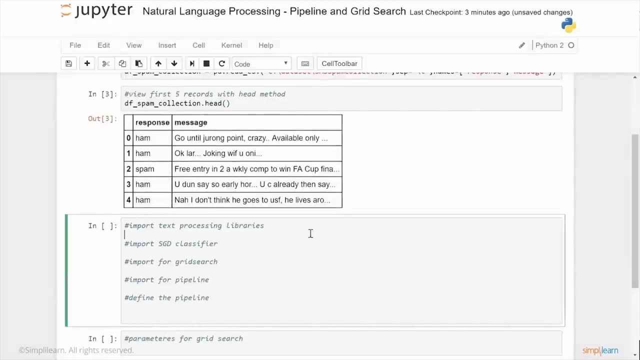 of the spam collection. The head method is used to view the topmost records in a dataset. Let's import scikit-learn specific libraries for text processing and creating the pipeline and performing the grid search. We will import counter vectorizer to tokenize the document. 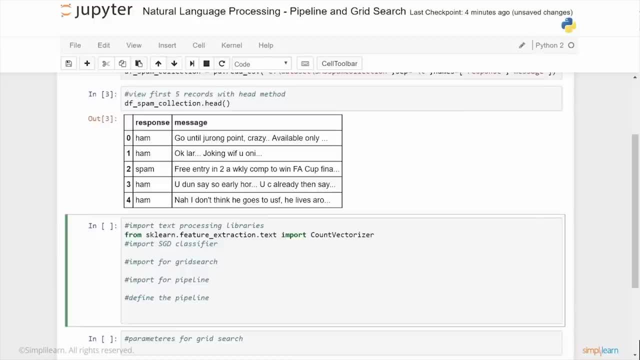 and convert the text into numeric values. Also, let's import TF-IDF transformer for TF-IDF transformation. Now import SGD classifier from the linear model. This is to classify the message in the dataset. Next, import grid search from the sklearn. 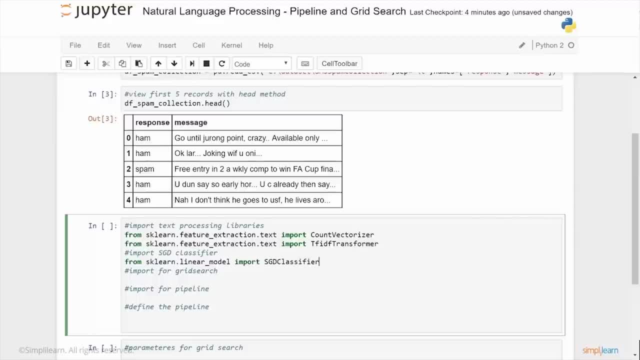 grid search class to perform the grid search. Finally, import pipeline from pipeline class. Let's import pipeline from pipeline class. Finally, import pipeline from pipeline class. Next, import pipeline from pipeline class. Let's create a pipeline by instantiating the pipeline class. 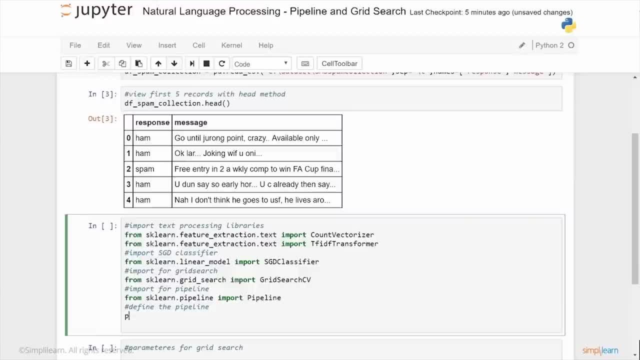 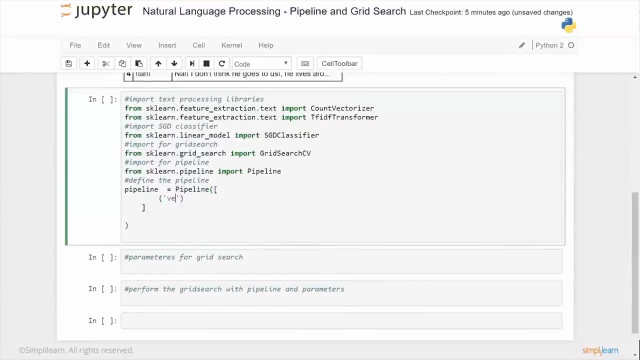 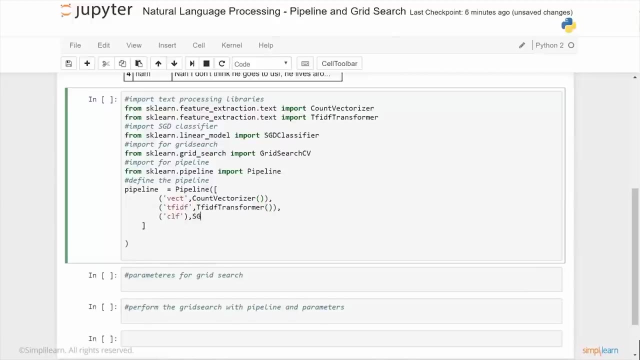 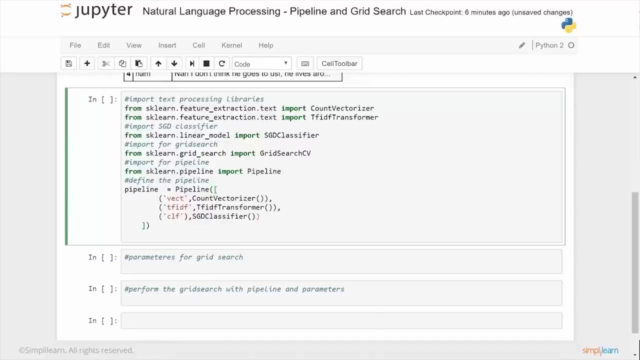 and passing, vectorize, transformed and model classifier as argument. The statement you see here helps create a pipeline for the entire text processing. Now let's define parameters for grid search. We are going to use the TF-IDF parameter to weigh the terms.